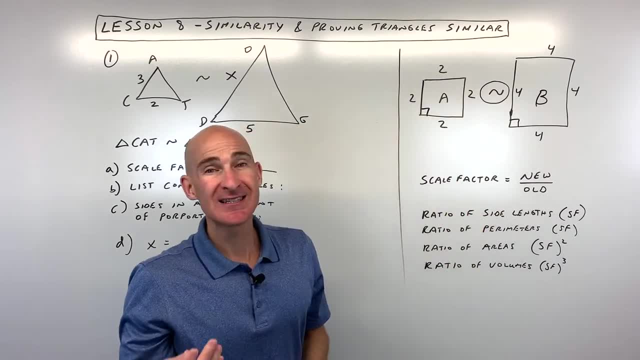 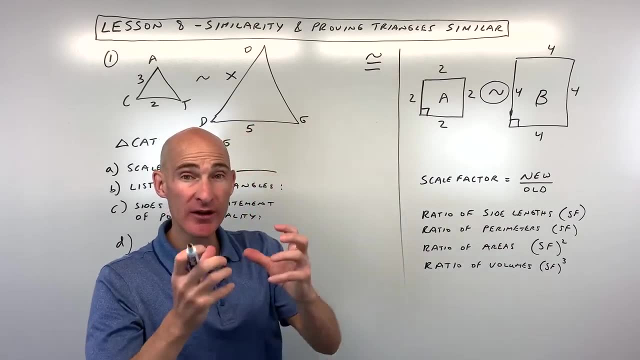 this little symbol, I should say, is the symbol we use for similar. Remember, when we talked about congruent, we used this sign where it was like the symbol here, with an equal sign underneath. that means congruent, like they're equal. When they're similar, we just use this symbol, that's. 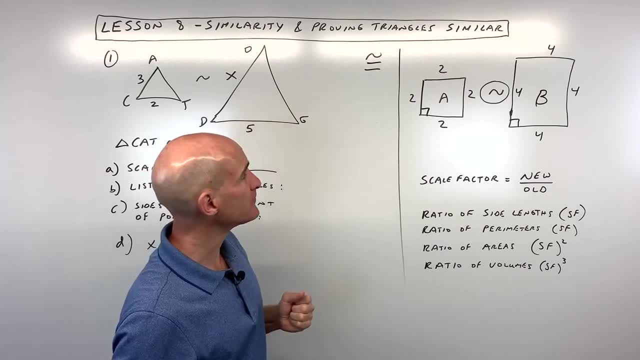 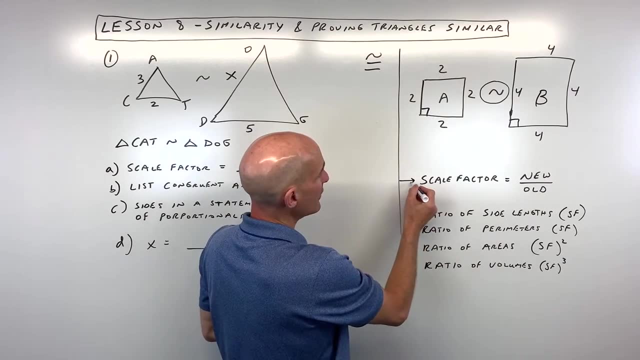 above that equal sign to show that the two figures are similar. Now the thing I want to show you is, if you're going from figure A to figure B, there's something called the scale factor. Okay, and what the scale factor is is like: what are you scaling it by? What are you multiplying it by to get to? 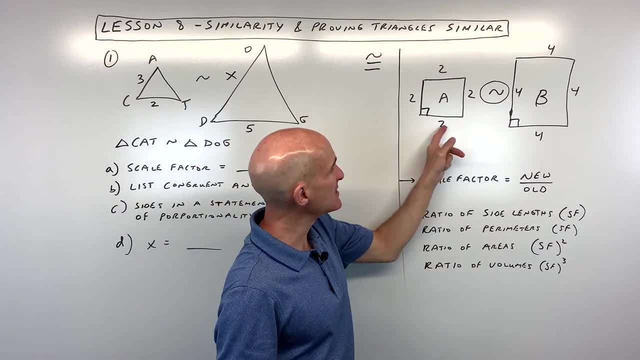 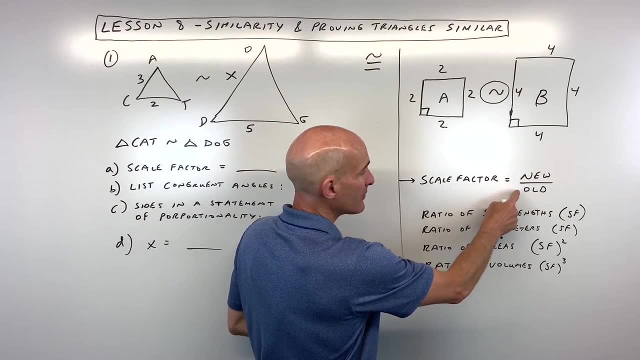 new side lengths. So for example, to go from 2 to 4, you can see we're multiplying by 2, but an easy formula to memorize here is: you take the new length divided by the old length. So if we're 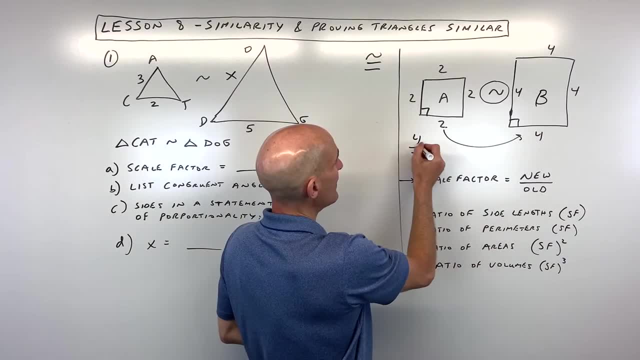 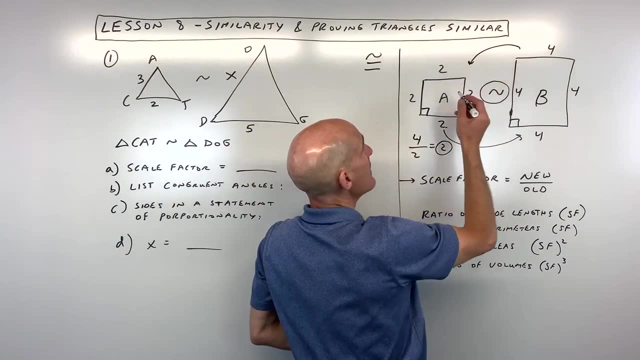 going from here to here. 4 is the new one. divided by 2, which is the old one, gives us a scale factor of 2.. Now say if we were going from figure B to figure A like this: now 2 would be the new side. 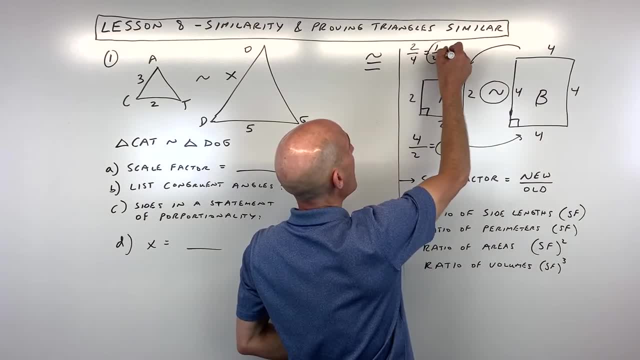 length 4 was the old one and you can see that's going to be one half. Notice that 2 and one half 2 is like 2 over 1, these are reciprocals of one another. So if you know the, 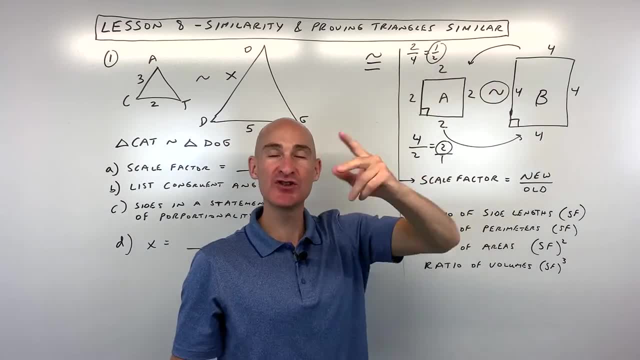 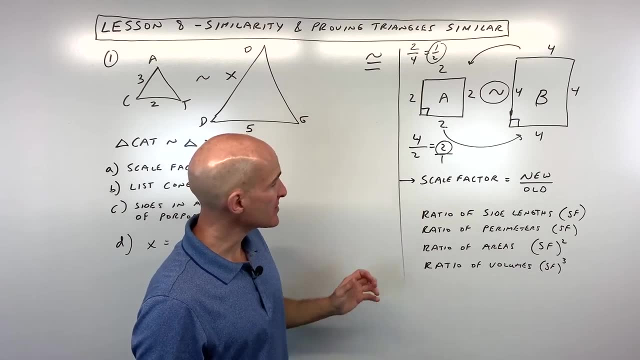 scale factor. going one way, you're automatically going to know it. going the other way, you just have to flip that fraction right Now. the other important thing that's really key to learn here is that when you're comparing side lengths, remember side length. that's like a one-dimensional right. 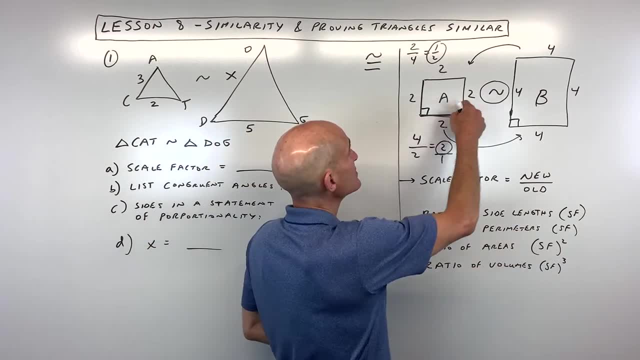 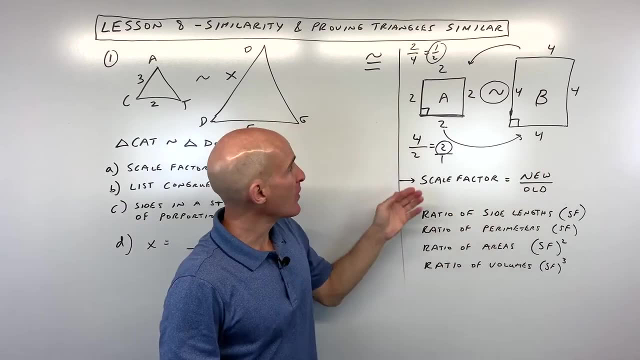 So if we were going to compare the ratio of the perimeters- like the distance all the way around the figure, because perimeter is also one-dimensional, it's just like length- the ratio of the two perimeters is going to be the same as the. 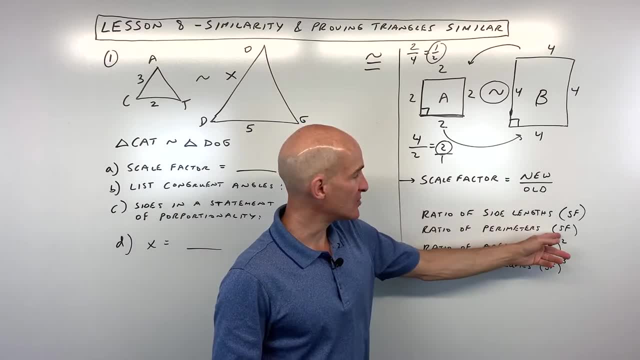 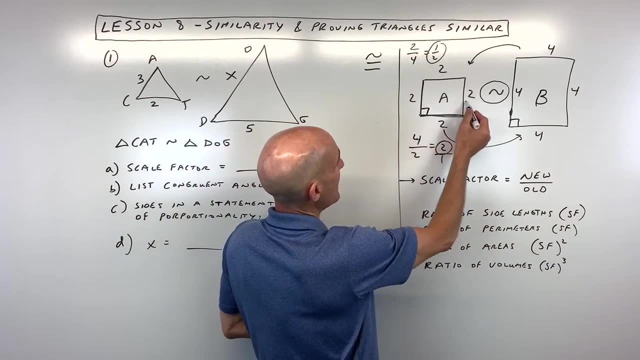 ratio of the side lengths or the scale factor. Okay, so I just kind of denoted this by sf or scale factor. So if you want to prove it to yourself, here you can see that the perimeter is 8, here the perimeter is 16, so you can see you're really multiplying by 2, same thing as the scale. 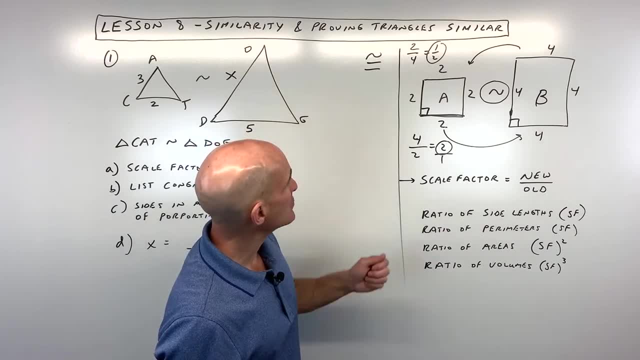 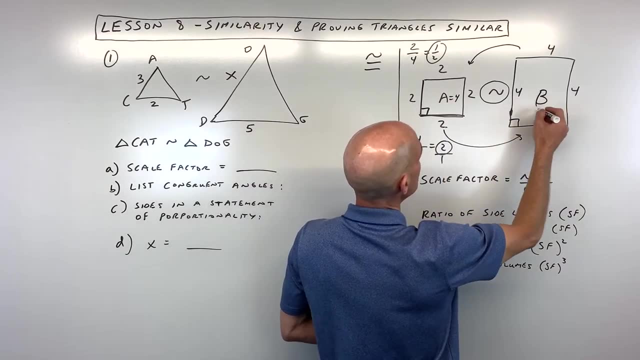 factor. Now, when you talk about area, look at what happens with area. So here we have 2 times 2,, which gives us an area of 4.. Here this one 4 times 4 gives us an area of 16, and what are we doing to get from 4 to 16?? 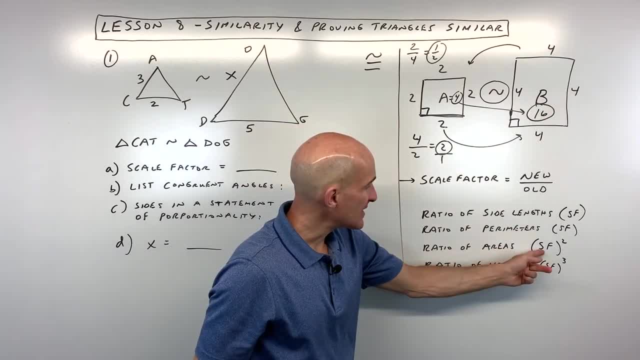 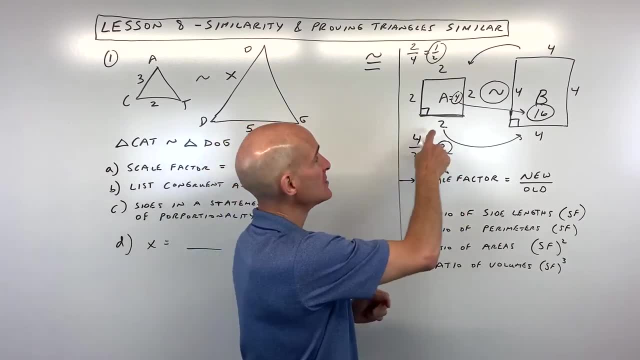 Well, you can see, we're actually multiplying by 4, which is our scale factor squared. Now, why squared? Well, remember, area is two-dimensional. it's like length times width. so if we double the length and we double the width, because we're multiplying by 2, and then by 2, right, that's 4, so it's like 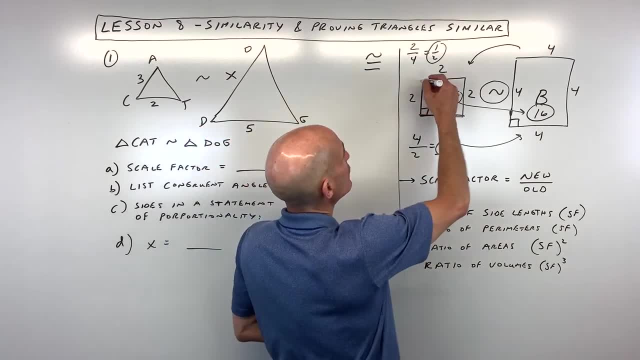 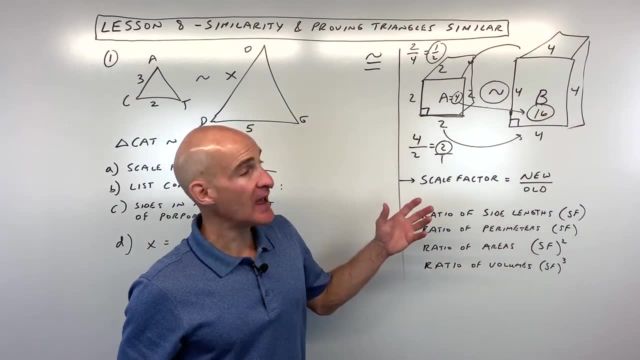 the scale factor squared. Now say, for example, we were to turn these into like cubes, Okay, like little ice cubes, little ice cubes, Little boxes like that. Now, what we're looking at is three-dimensional. Volume is length times. 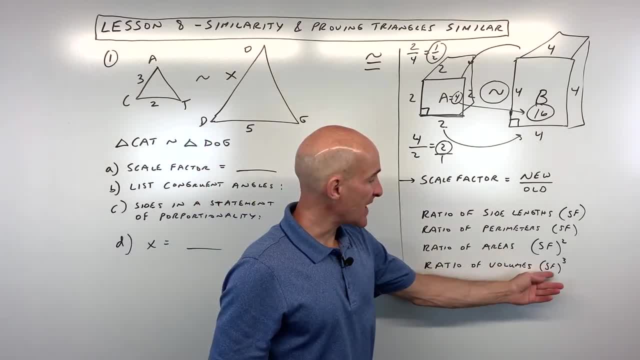 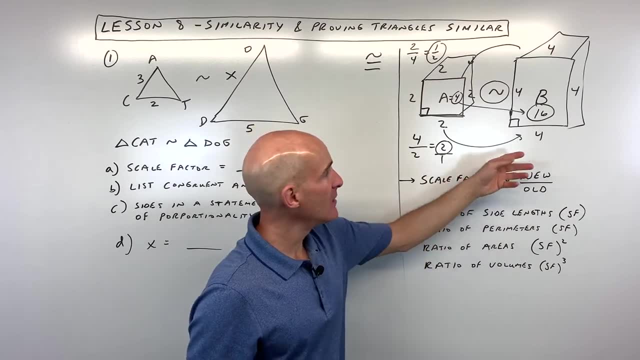 width times height. so when you compare the volumes, it's actually going to be the scale factor to the third power, the scale factor cubed. So here we have 2 times 2 times a height of 2, that would be 8.. 4 times 4 times 4, that's 64.. 64 is 8 times larger, right? So that's important. 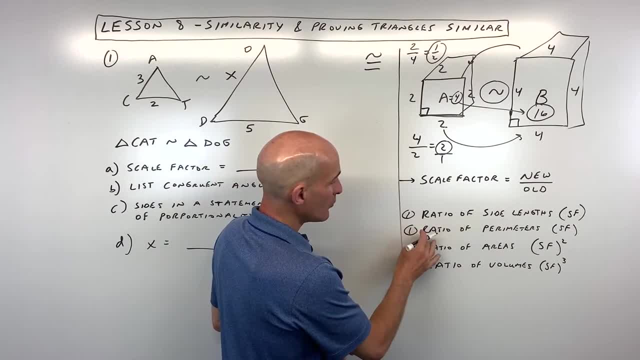 to remember. So sometimes I just like to think of scale factors like one-dimensional. perimeter that's one-dimensional, so that's just the scale factor. Area is two-dimensional, so that's the scale factor squared, and then the ratio of the volume is the scale factor cubed. So let's do 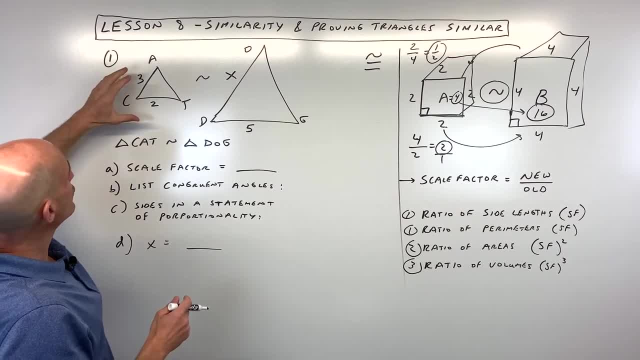 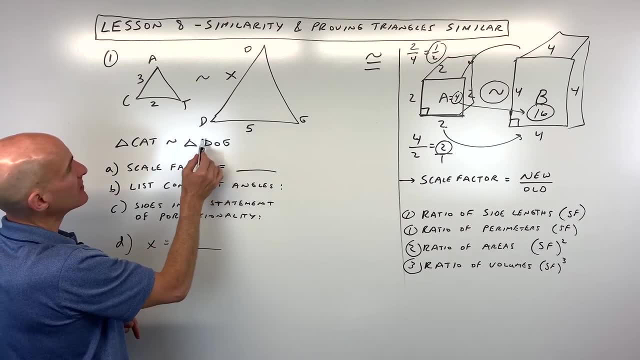 number one here. See if you can do this problem. So say, for example, we're going from this triangle cat- okay, c-a-t. and we can see that it's similar to triangle dog- okay, d-o-g. Now remember just: 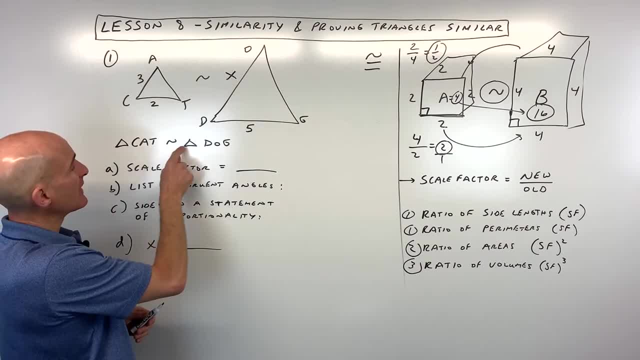 like when we learned about congruent triangles, in this similarity statement the letters that match up are going to be the corresponding vertices. So c matches with d. that means angle c is congruent to d, a with o, t with g, like that Also, you can see that side c-a is going to match up with side d-o. 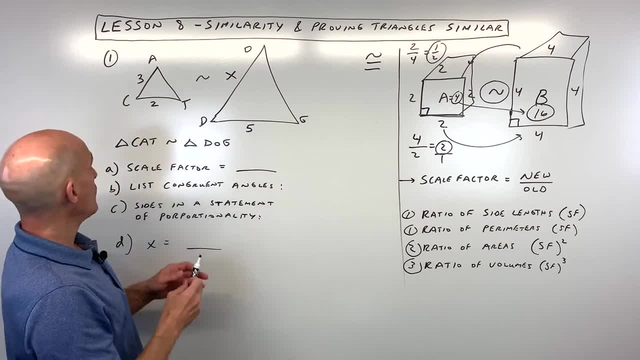 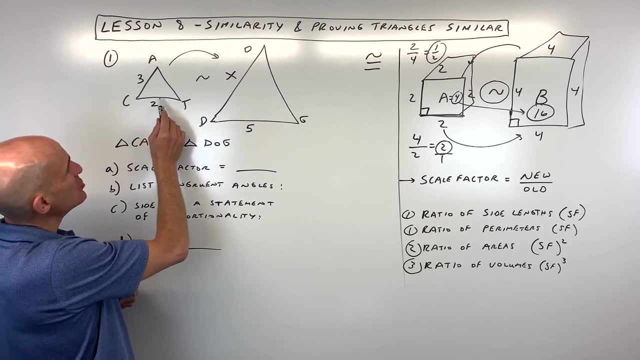 see first and second, first and second, etc. So here it's asking us: what's the scale factor from cat to dog? Well, you can see that 2 is turning into 5, that's two and a half times larger. 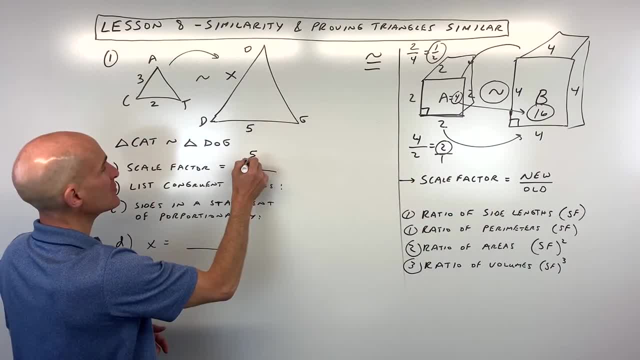 Or, if you want to use our formula here, scale factor is new, which is 5,, divided by old, which is 2,, which gives us a scale factor of 2.5, or you can just leave it as a fraction. 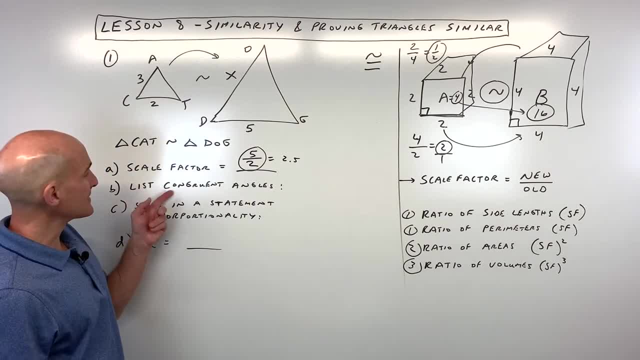 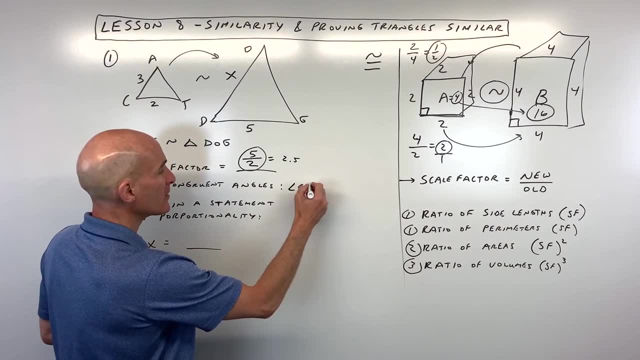 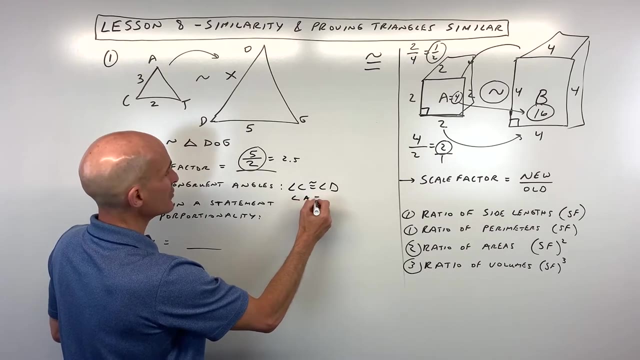 Five halves Now here. part b says list the congruent angles. So we kind of talked about that already. You can see angle c matches with angle d, but we'll just write it a little bit more formally. more formal here: Angle c is congruent to angle d, angle a is congruent to 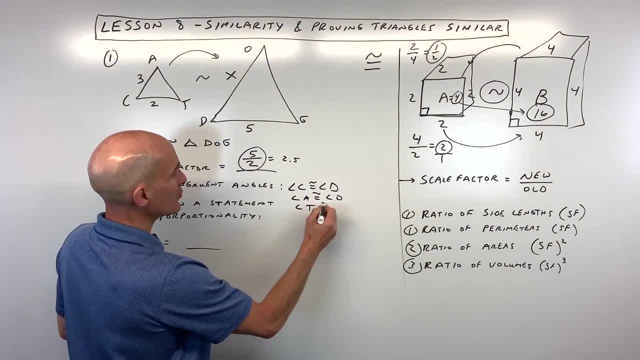 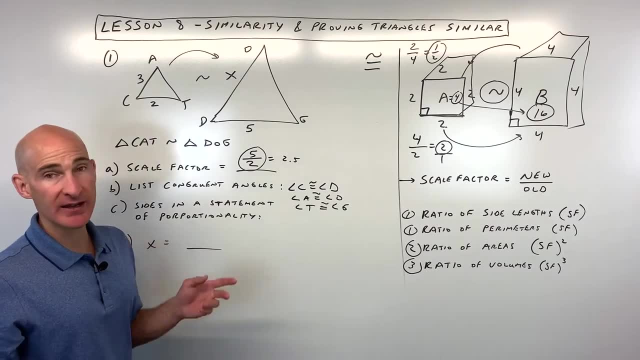 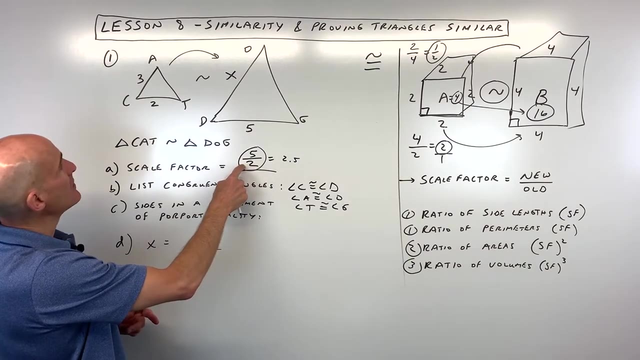 angle o and angle t is congruent to angle g. Okay, so cat and dog. And then here it says: list the sides in a statement of proportionality. Now, what does that mean? a statement of proportionality? Well, remember how we said: the ratio is 5 to 2? Okay, five halves. And remember how we said that. 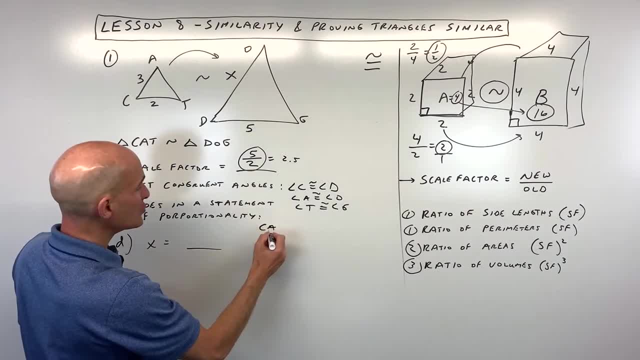 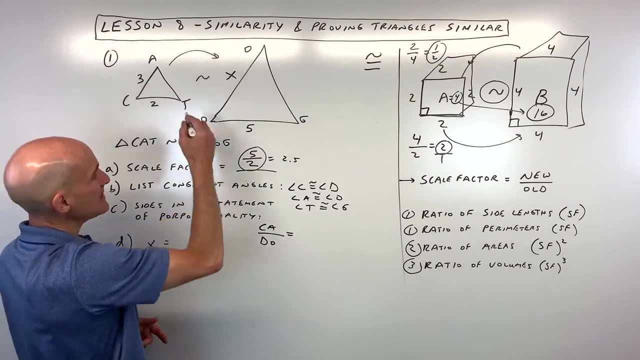 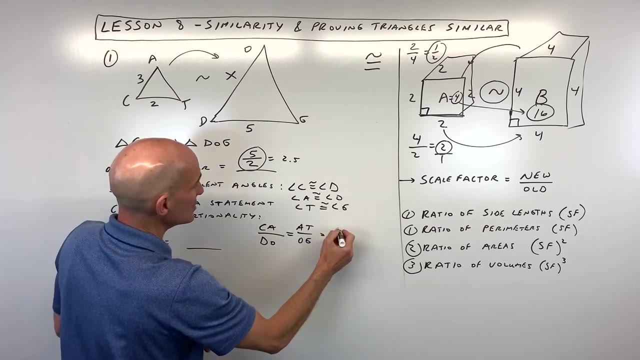 ca corresponds with do. So what we have is the ratio of ca, this side to do. this side is going to be in the same ratio as at is to og, as ct is to dg, So all these are going to be the same. 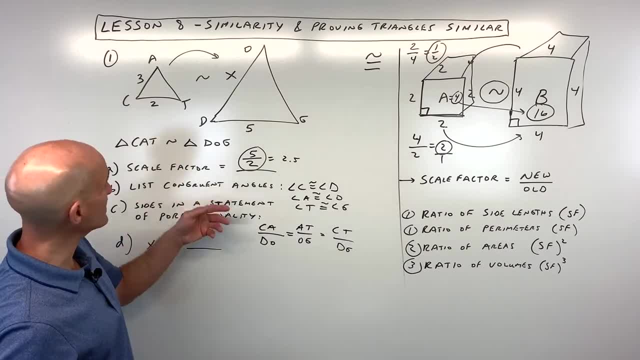 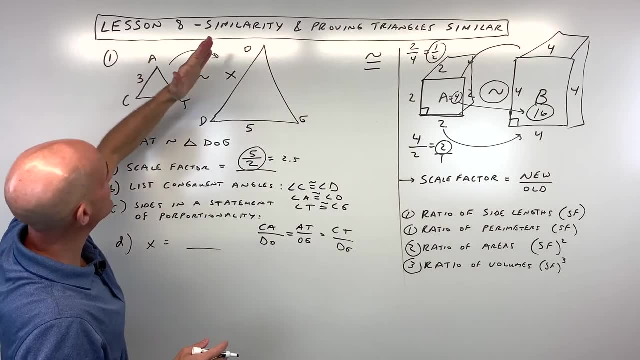 5 over 2, that same ratio, Right. Or in this case, we did ca to do. that's going to be 2 to 5.. The main thing you want to pay attention to is that you keep the order the same. So I do this side is to this side I want. 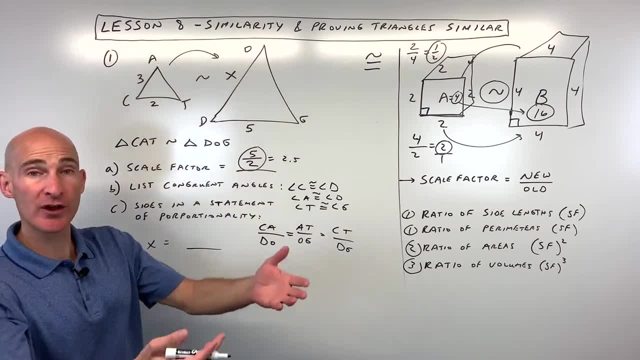 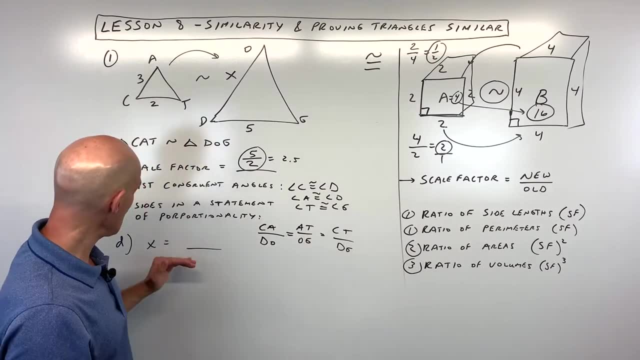 to do. this side is to this side, left to right, left to right. Or you can do it the other way, right to left, right to left. You just want to keep it consistent. All these ratios are going to be the same when the figures are similar. And then the last part. here it says: well, 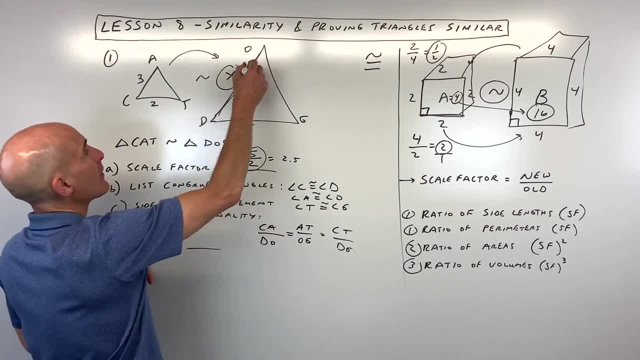 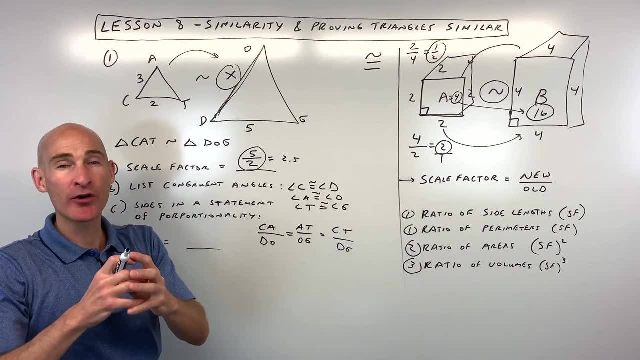 what is x equal to? So what is this side length right here? Well, we don't really know right. But what we can do is we can form a proportion. Remember similar figures. they're proportionally larger, proportionally smaller. Of course, it could be the same. 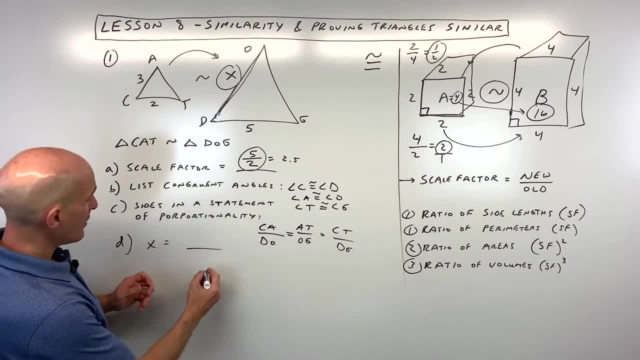 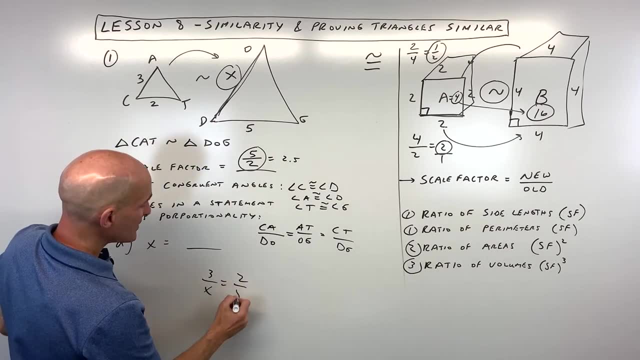 then it would just be like a one to one proportion. But let's go ahead and make a proportion here. So we have 3 is to x as 2 is to 5.. Now notice how I kept that order. the same I did: left is to right, left is to right. Okay, Or I could have done it the other way. 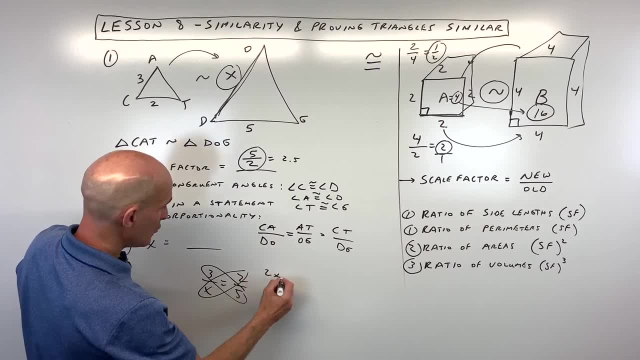 We'll just go ahead and cross multiply, So that's going to give us 2x equals 15.. And if we divide both sides by 2, that's going to come out to 7.5. Or you could leave it as 15.5.. 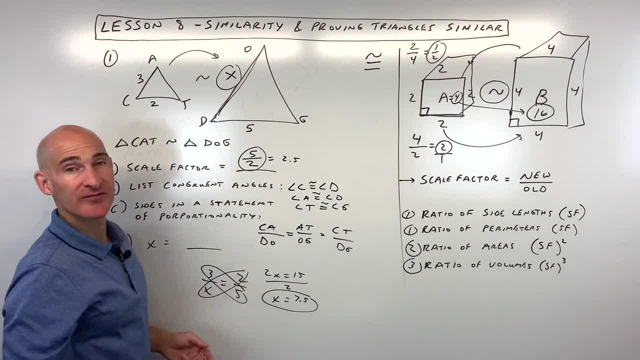 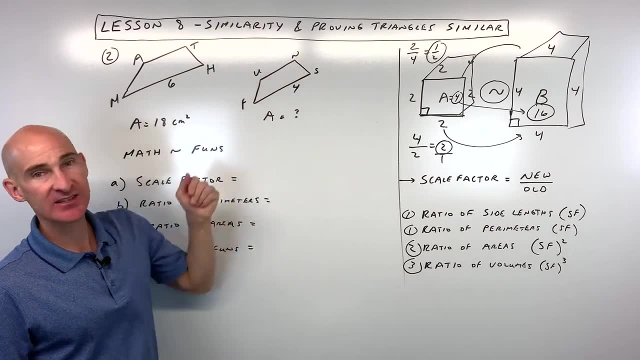 And that's going to be the length of this side here. Okay, See, if you can do example number 2: here We have m-a-t-h and f-u-n-s, So like math and funds, Okay. So here we have: math is similar. 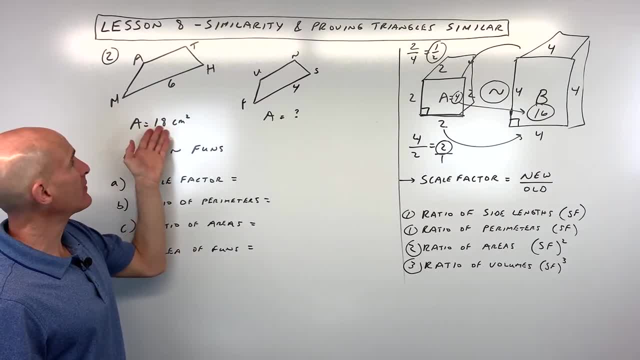 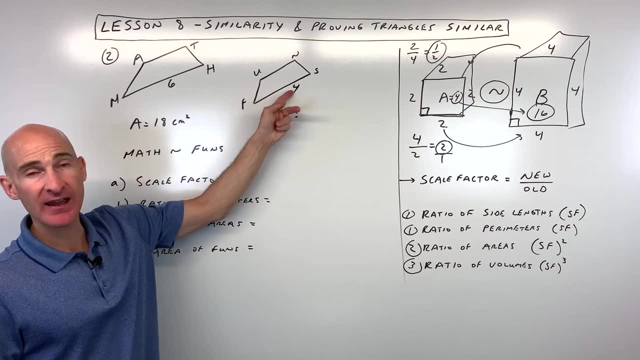 to funds, And they're giving us the area of this first figure, math, But we want to figure out eventually the area of this second figure. okay, f-u-n-s, And they give us the side lengths, Okay, So what do you think for part a, the scale factor? So what's the scale factor from? 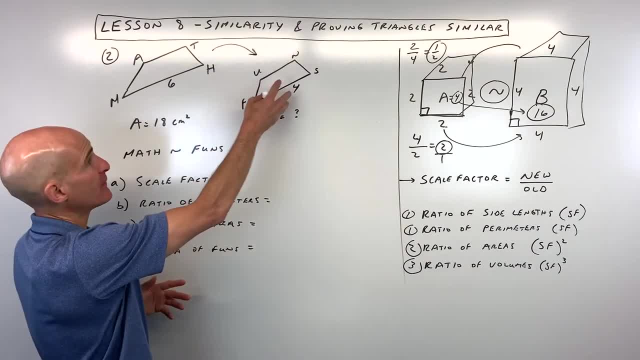 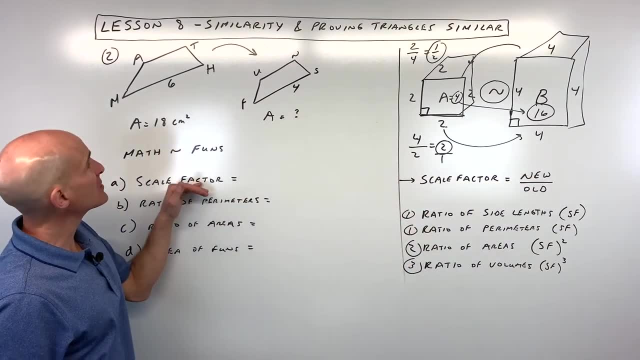 math to funds And normally in these problems they'll tell you: is it math to funds or funds to math? And remember, the order is important because when we do the scale factor we're thinking new over old. So what do you think for this one? Well, the new one is 4.. The old 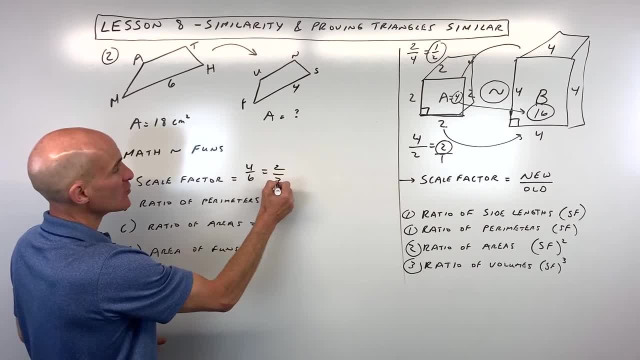 one is 6.. So it looks like it's going to be 4 over 6, which we can reduce by dividing these both by 2 to get a scale factor of 2 thirds. Okay, What do you think for part b, the ratio? 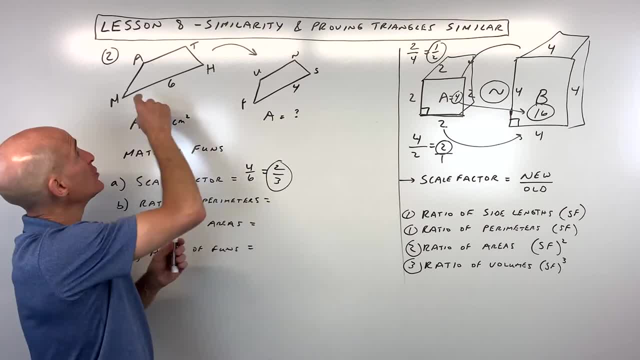 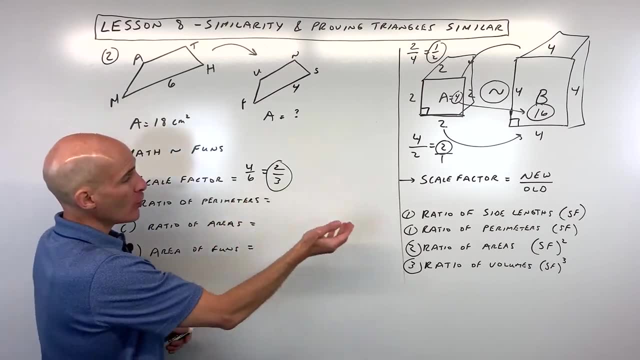 of the perimeters, the distance all the way around. Well, it's interesting. We don't actually know all these side lengths, So it's not like we can like figure out the two perimeters and then write it as a ratio. But we know that the ratio of the perimeters is the same. 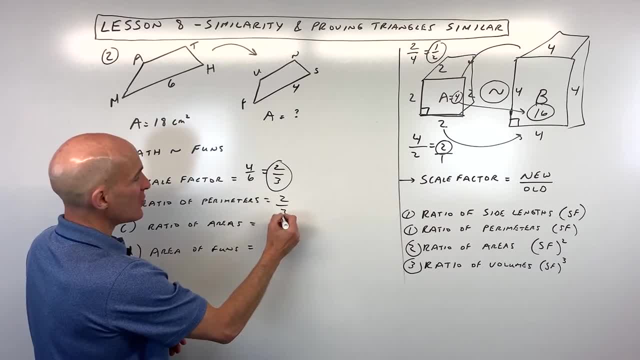 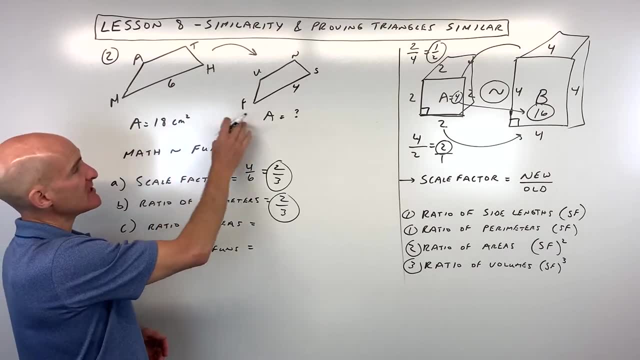 as the scale factor. So that means the ratio of perimeters is also 2 thirds. How about part c, the ratio of the areas, the inside of these figures? We know this area is 18.. We don't know the area of this one, so we can't again just write it as a ratio, But remember. 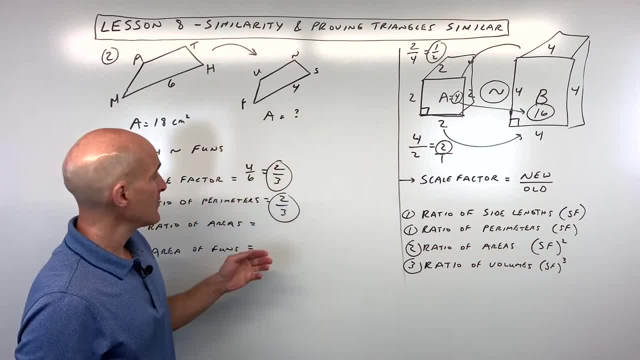 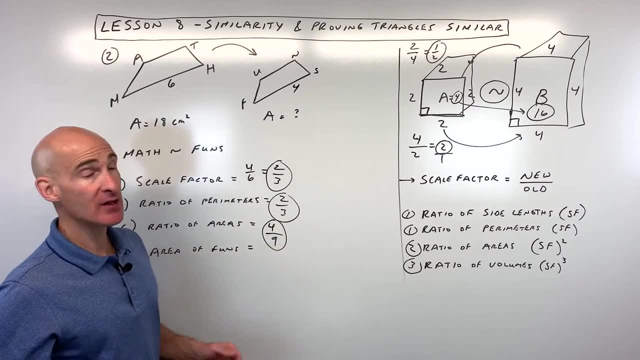 how area is two-dimensional and we said it's the scale factor squared. So 2 thirds squared. if we square two, that's 4.. If we square 3, that's 9.. So that's a ratio of 4 to 9, comparing the areas. And then now 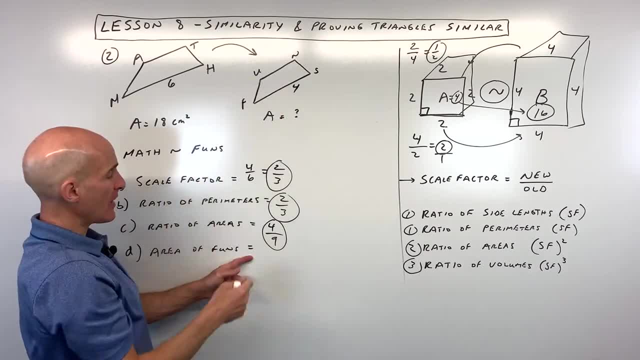 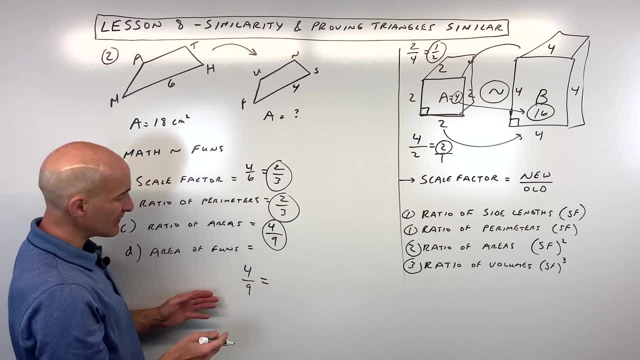 this one. what's the area of the second figure, FUNS? Well, what we can do is we can make a proportion. We know the ratio of the areas is 4 to 9. And this is important. This is where students sometimes make a little bit of a mistake. See how I'm comparing this: 4. 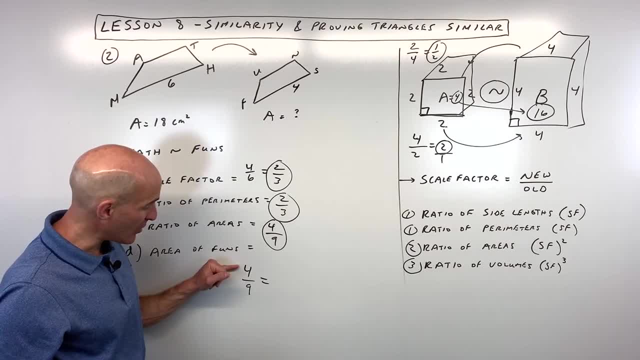 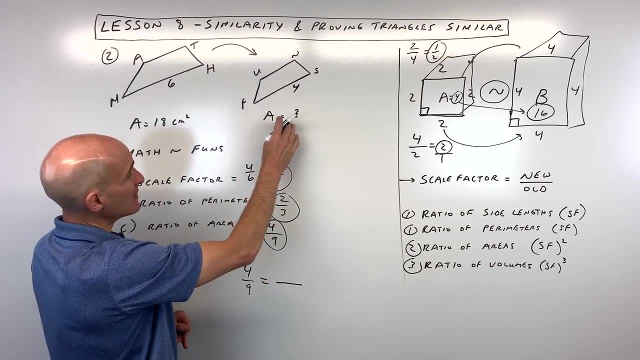 to 9?. 4 is smaller than 9.. That means we're comparing the smaller area to the larger area, right? Or you could think of: okay, this one's smaller than this one, right? So we're doing, this is going to be a, or we'll just call it x. 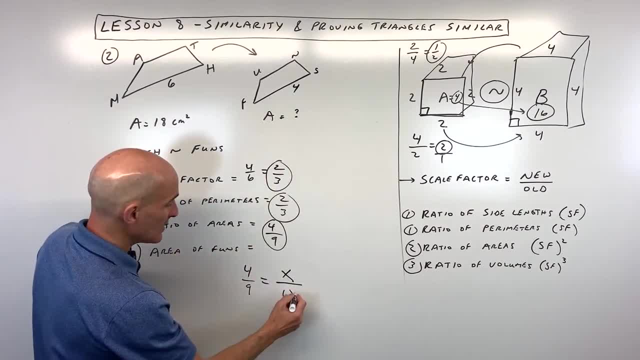 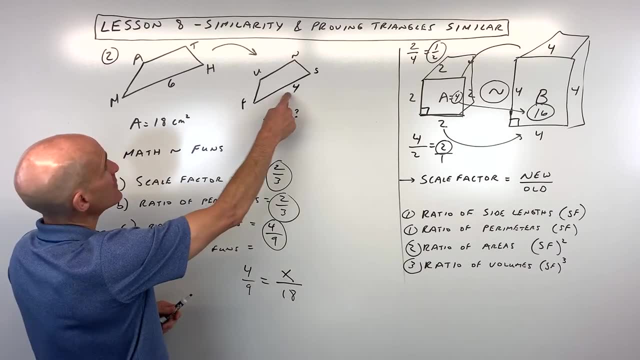 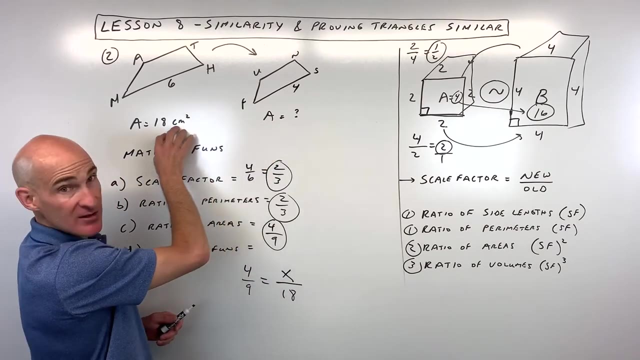 we don't know this area to this one here, which is 18.. So does that make sense? My figures are not super obvious here, but you can usually tell which one is smaller. You can see 4 versus 6.. This is smaller. So we've got small to large, small to large. right, The smaller area to this larger. 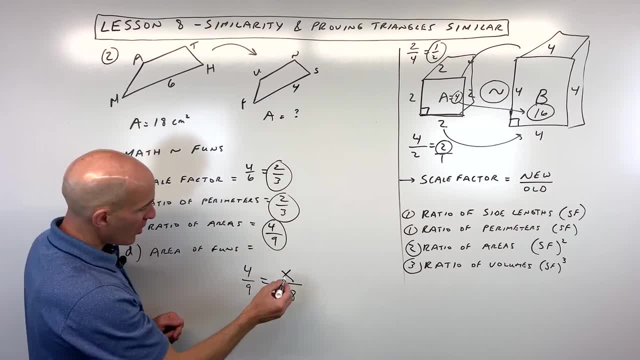 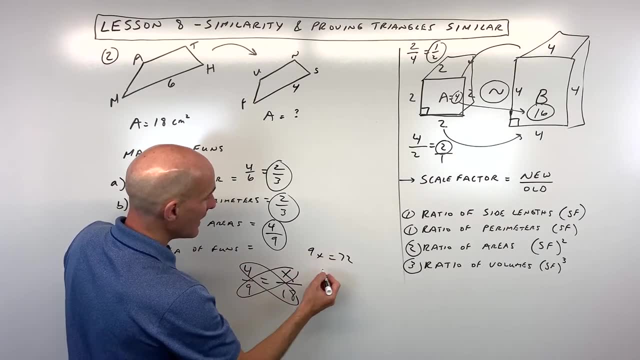 area. You want to keep it in the same ratio, otherwise you're going to get the wrong answer. the same order. So here we have: 9x equals 72. So if we just use our cross product and divide both sides by 9,, 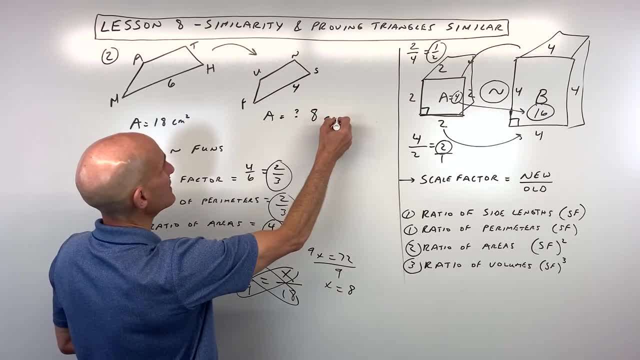 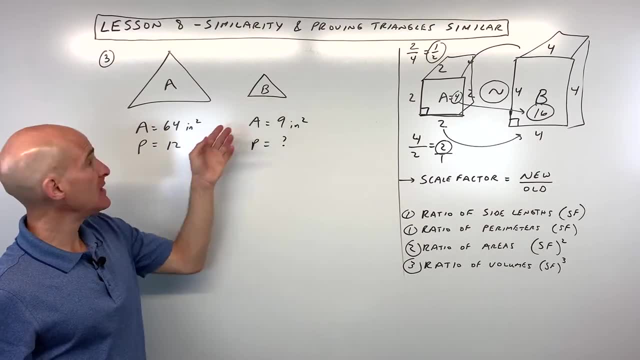 that's going to give us 8.. So this area is 8 centimeters squared. For example, number 3, we're given the area of figure A and the area of figure B, and we're given the perimeter of figure A, We're trying to find the perimeter of figure B. So what do you? 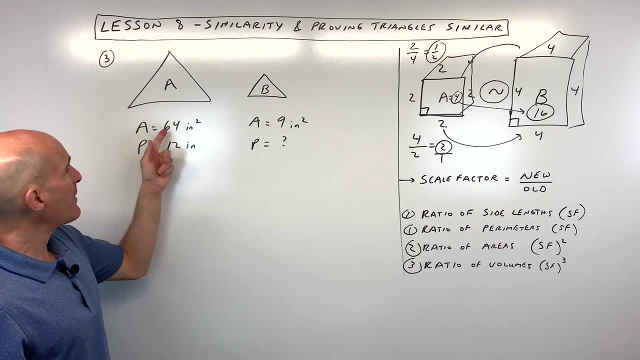 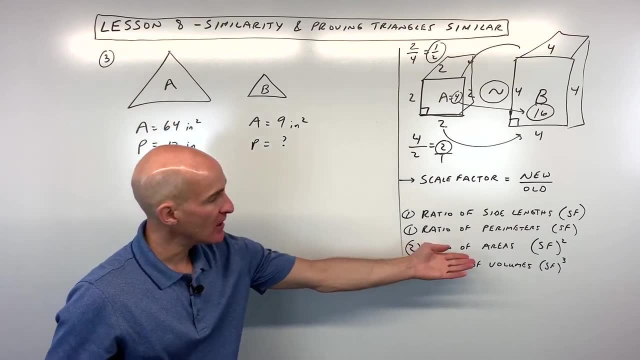 think you would do on this one. Well, let's start off by writing the areas as a ratio. So we have 64 is to 9.. Now this is the ratio of the areas. Remember, the area is like the scale factor squared, If we want. 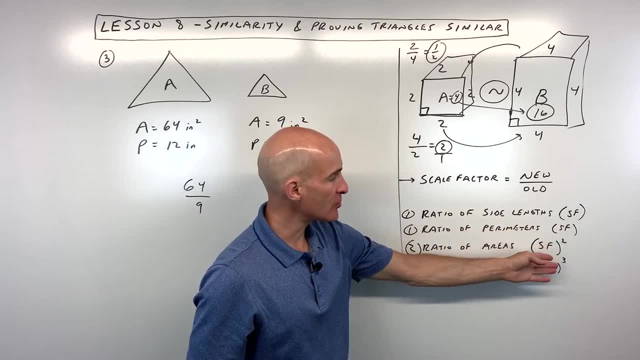 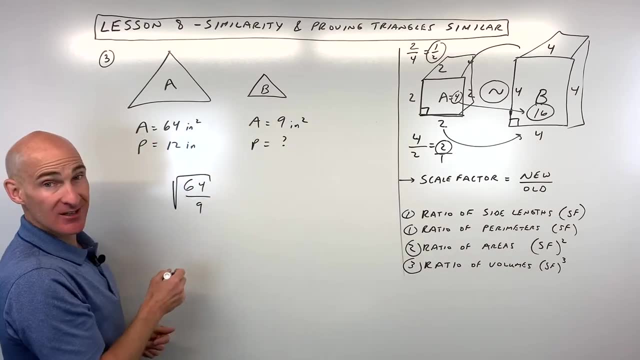 to find the ratio of the perimeters. see how this is the same as the scale factor. How do we go from the scale factor squared to just the scale factor? Well, we can take the square root, And when you take the square root of a fraction, it's like you're taking the square root of the numerator. 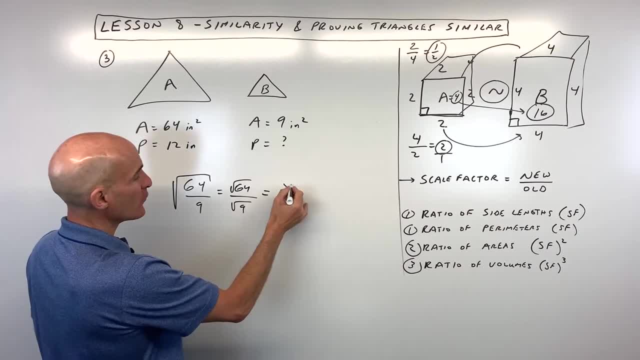 and the square root of the denominator. You can do it separately, like that: Square root of 64 is 8.. Square root of 9 is 3.. Now we know the ratio of the side lengths and the square root of the denominator. 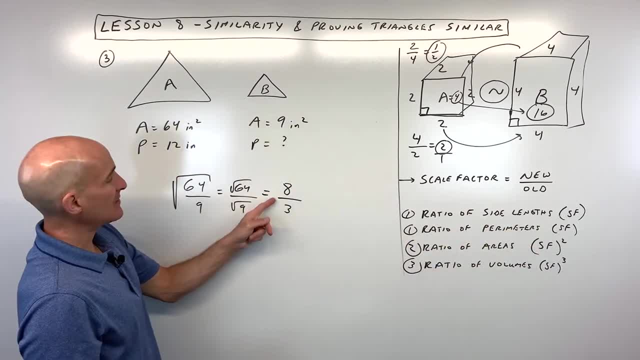 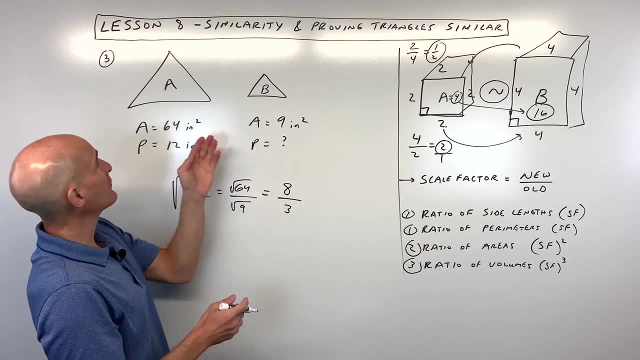 As well as the ratio of the perimeters. Now notice 8 is larger than 3, right, Just like this area 64 is larger than this area 9, so we have large to small, or you can think of left to right, So here, 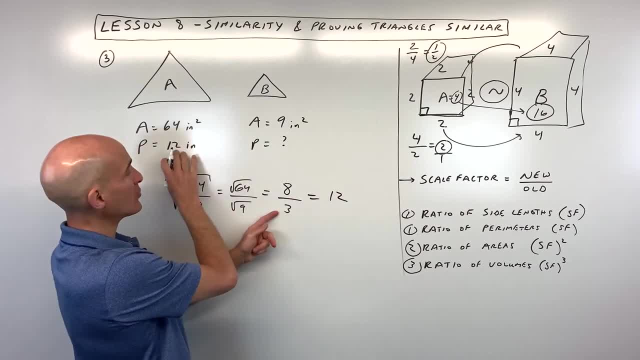 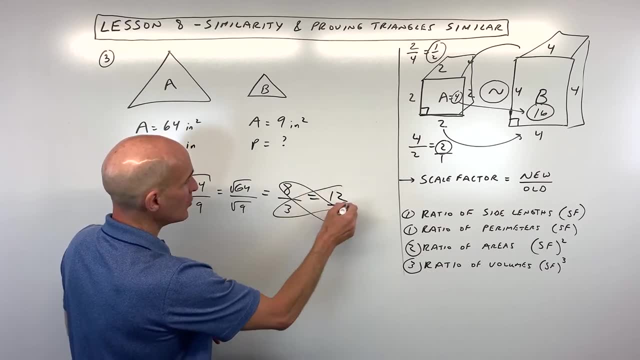 we have left to right is the same as the perimeter 12 left. so this perimeter here, right. Okay, so we can just cross. multiply now We have: 8x equals 36, divide both sides by eight and that comes out to 36 eighths which, let's see, is 4.3 of 8.5.. So we have those two energies here. I'm going to 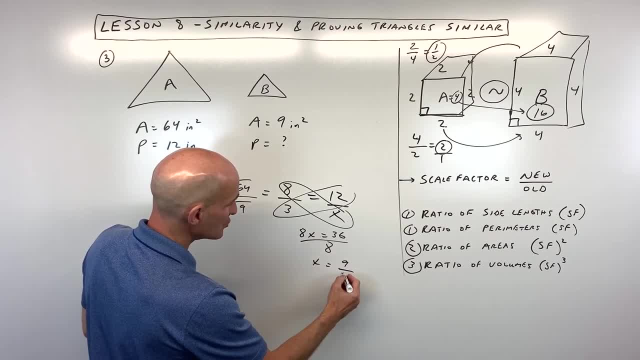 write both sides by 8, and that comes out to 36 eighths, which let's see: 4, 6, 9,, 8,, 9, and 8.. 4 goes into here 9 times. 4 goes in here 2 times. 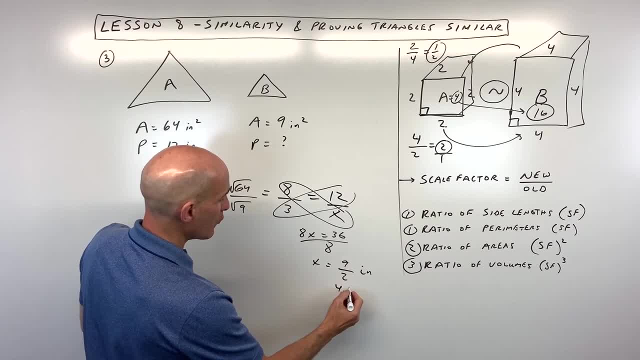 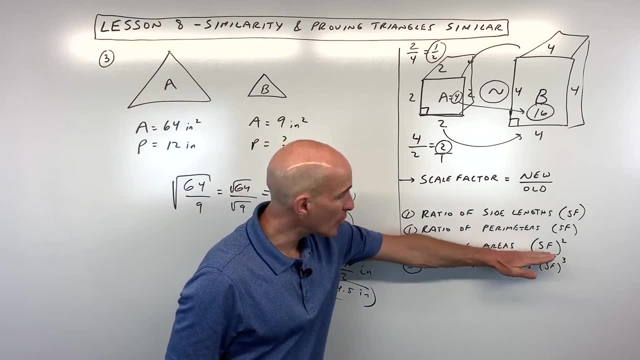 So it's 9 over 2 inches, or you could say 4.5 inches is the perimeter for B. So the key here is figuring out what are they giving you. If they're giving you the ratio of the volumes, that's the scale factor cubed, you would have. 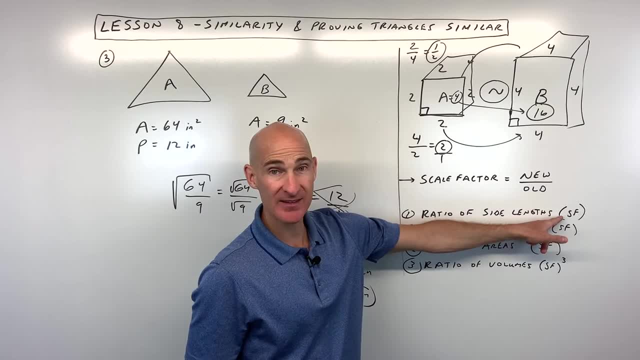 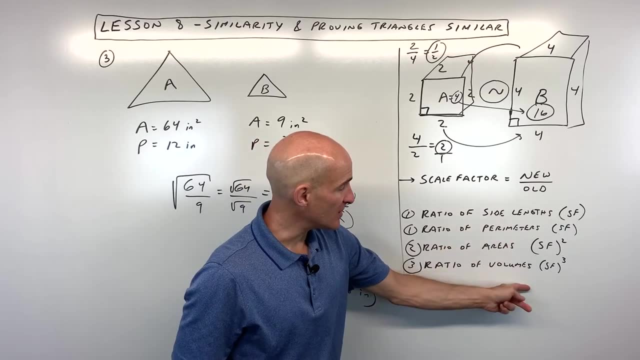 to take the cube root to get back to the scale factor, which is going to be the same as the ratio of the perimeters. If they gave you the ratio of the perimeters, you could then cube it to get the ratio of the volumes. 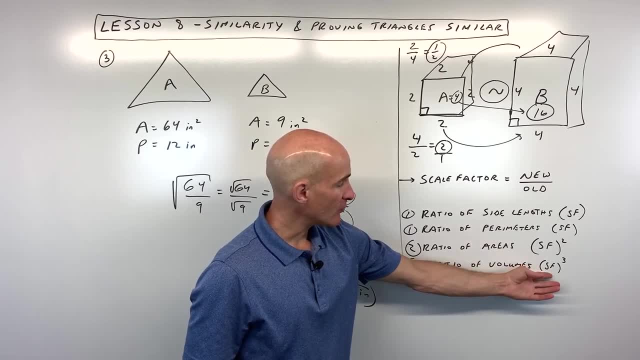 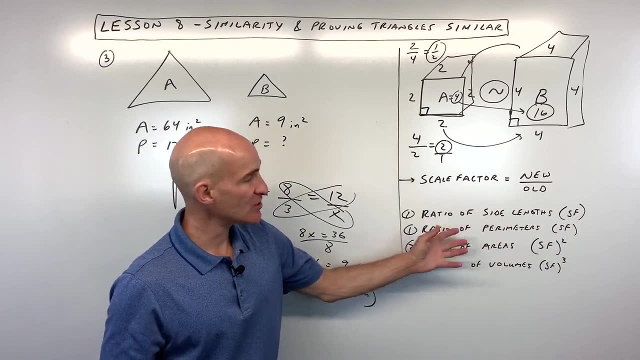 Or if you wanted to find- let's say they gave you the volume ratio- you could take the cube root to get back to the scale factor and then square it to get the ratio of the area. So you always want to kind of think: is it 3-dimensional, 2-dimensional, 1-dimensional? 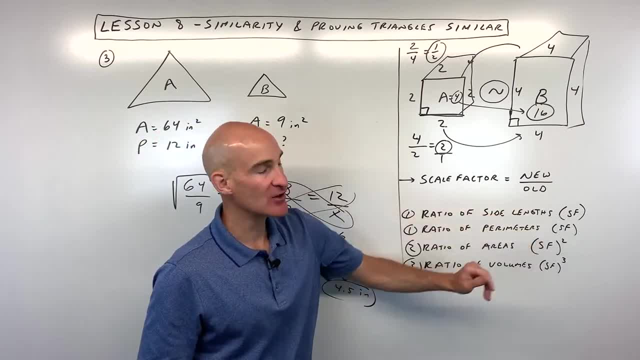 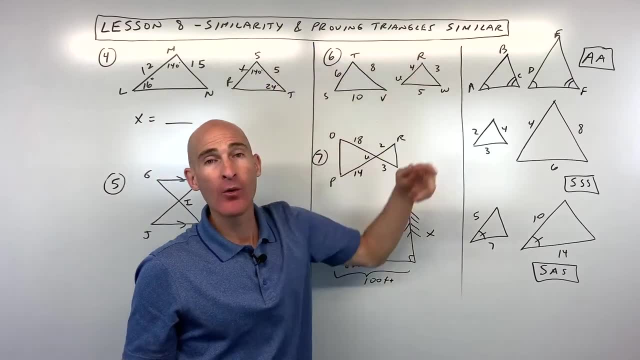 and how do I get back to the basic scale factor and you can take it from there. Okay, now we're switching gears, talking about how do we prove triangles are similar. Well, in an earlier lesson, remember how we showed triangles. 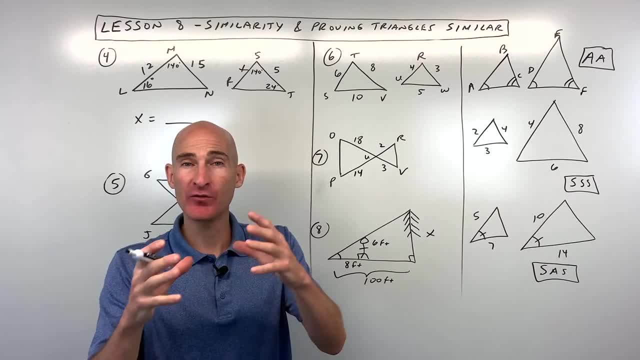 Triangles are congruent, meaning they're exactly the same. if we cut one out and we match it with the other one, it's going to be a perfect match. And remember there was five different ways to prove triangles are congruent, right. 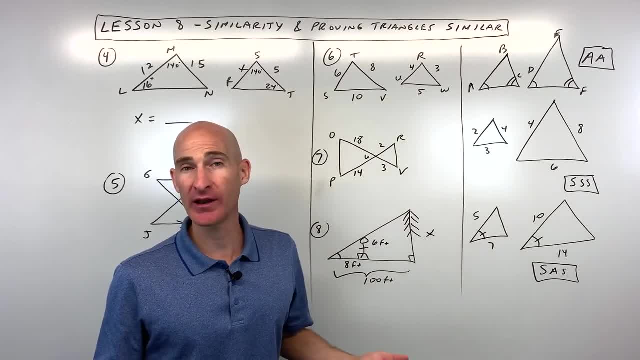 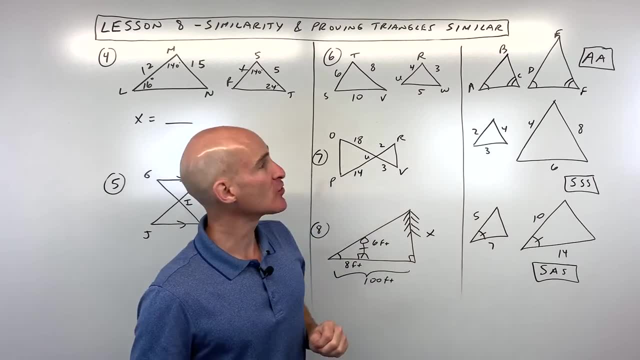 We talked about side-side-side, side-angle-side, angle-side-angle, angle-angle-side and hypotenuse leg, But here to prove triangles similar, we only have three methods, so it's a little bit easier to memorize. We've got the angle-angle, the side-side-side and the side-angle-side, so let me show you. 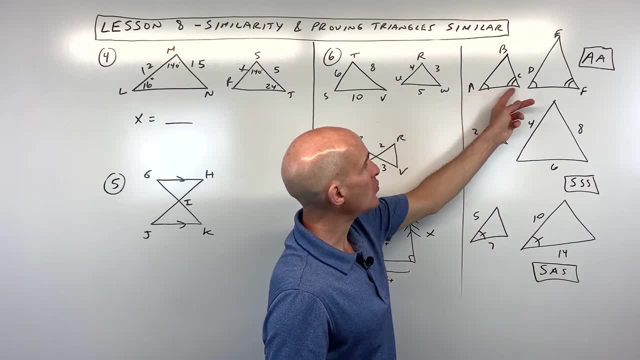 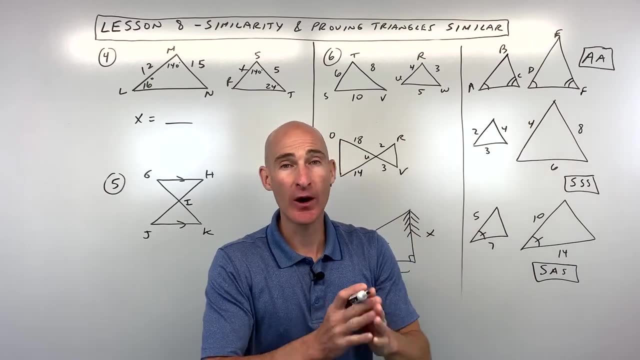 what that means. So for this one here, if you can show that two angles are congruent, then you can prove triangles are congruent. So if two angles in one triangle are congruent to two angles in another triangle, then we know that the triangles are similar. 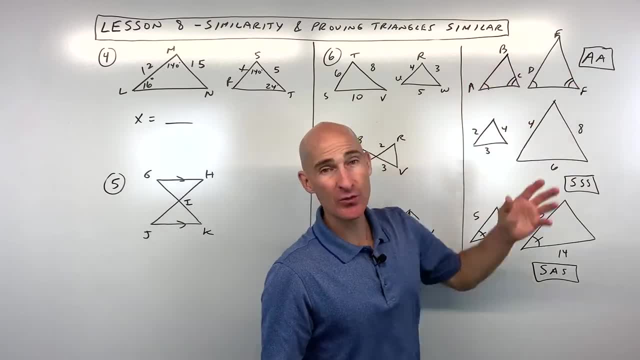 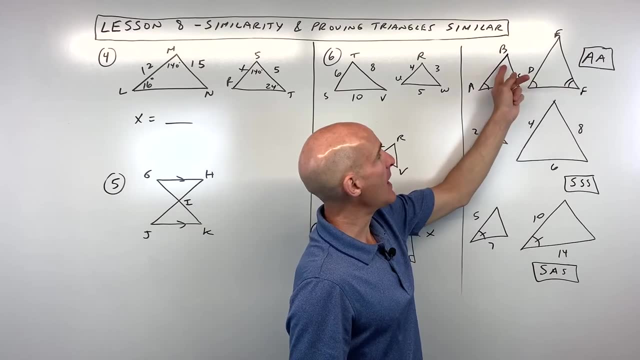 Now, why is it important that they're similar? Well then, we can form a proportion, we can solve for the missing side lengths, etc. Now, if two of the angles are congruent, okay, then automatically the third angles will also be congruent. 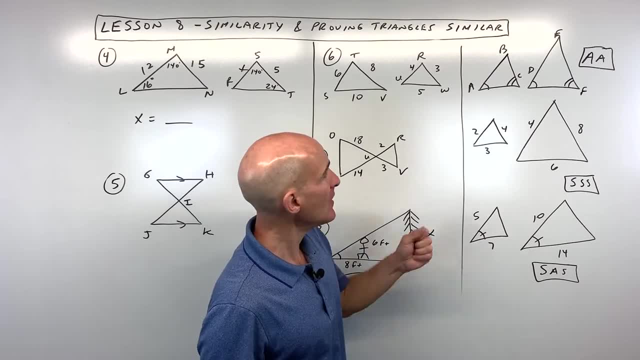 Okay, so that's just interesting to know. that's called the third angles theorem. So angle-angle is pretty simple. show two angles are congruent to two angles and then you can prove the triangles are similar. you just say angle-angle similarity. 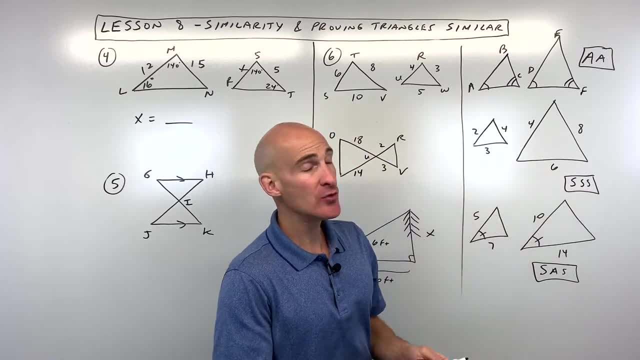 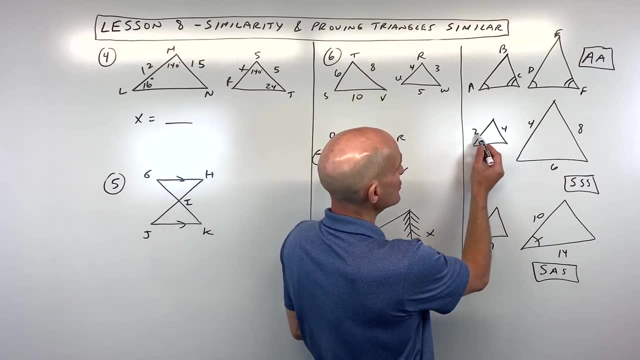 For this one. here, though, the side-side-side, what you want to do is you want to show that the ratios of the corresponding sides are in the same ratio. So for example here see: two to four, that's one half. four to eight, that's one half three. 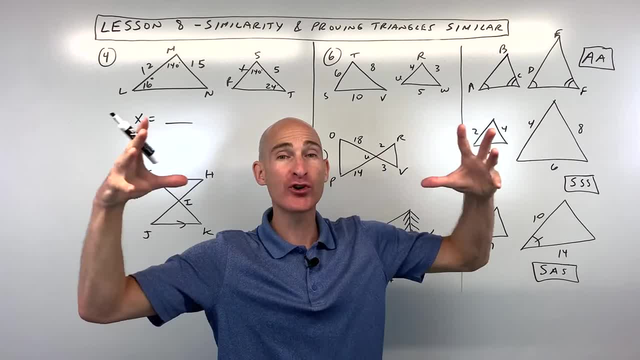 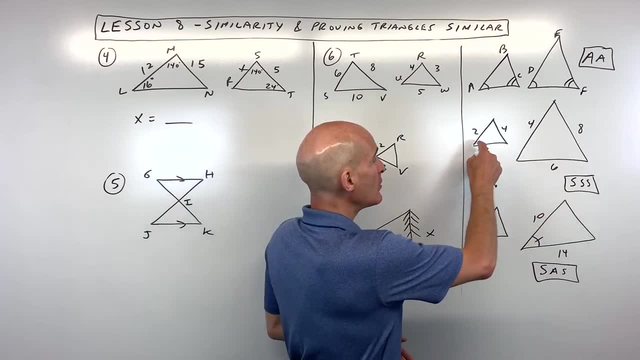 to six. that's one half. they're all in the same ratio, so it's proportionally larger. Now, once you prove that the triangles are similar by the side-side-side similarity, why is that important? Well then, we know that the corresponding angles, the angles that match up, are going to be: 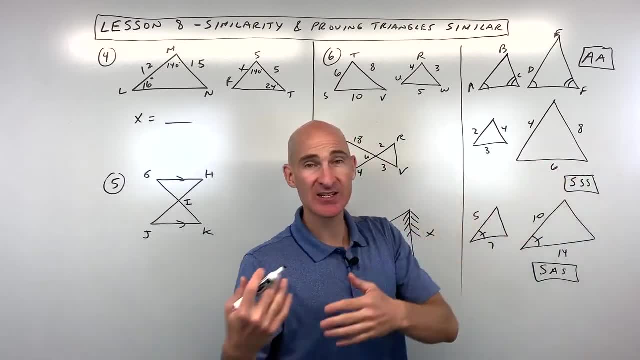 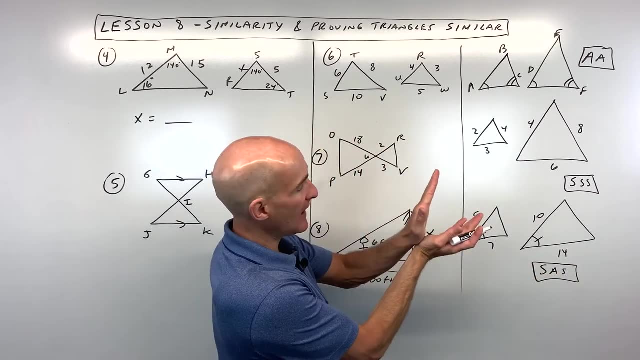 congruent, So you can, once you prove that you can take it a step further. And then for the last one, the side-angle-side, notice how that A is in between the two S's. we call that the included angle. 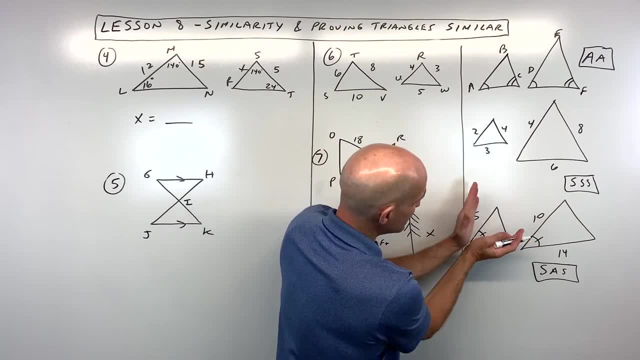 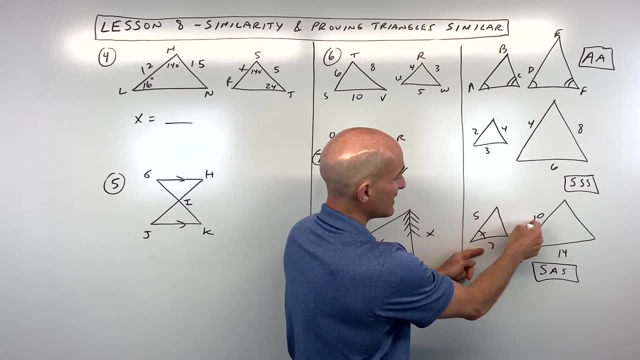 And if the included angle is congruent- see, these are the same and the sides that make up that angle, the two sides on either side of that angle, if they're in the same ratio, see, in this case, five to ten, that's one half. seven to fourteen, that's one half, they don't. 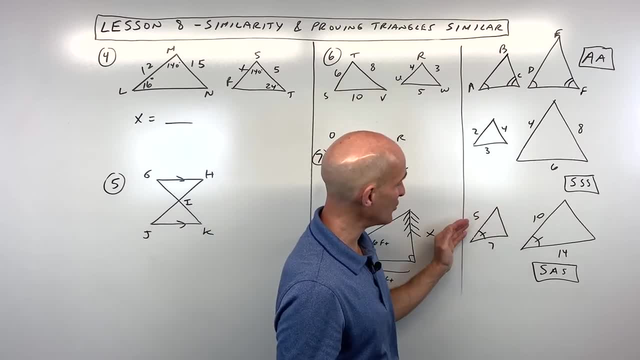 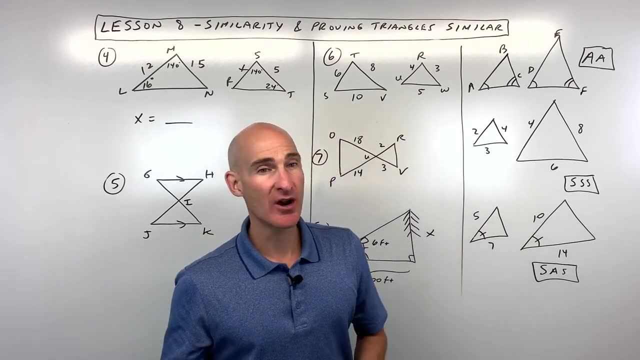 have to come out to one half. that's just a coincidence. but as long as they're the same ratio, like if it was one to three, one to three, Okay. So if the angle between is congruent, then we know that the triangles are similar and 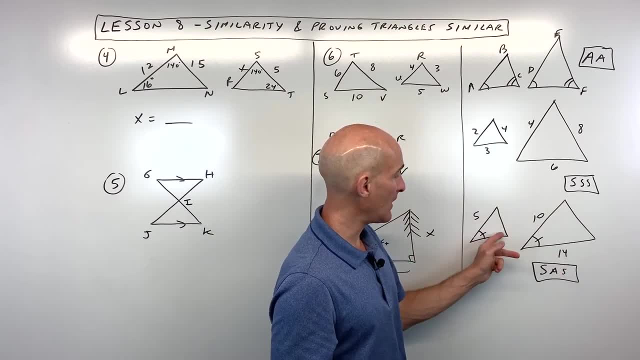 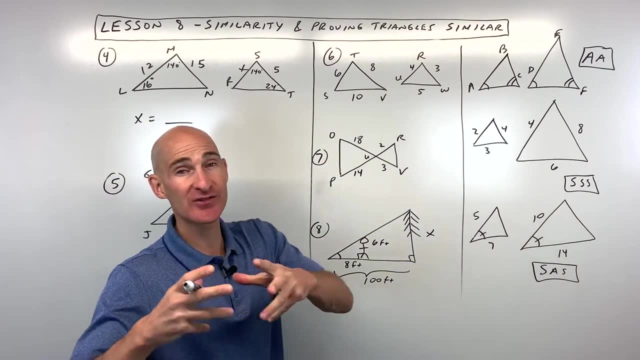 then the corresponding sides are going to be proportional, then that same ratio and the corresponding angles are going to be congruent. okay, So just remember: with similar triangles or similar figures, the angles are the same. it's the sides that are proportional. 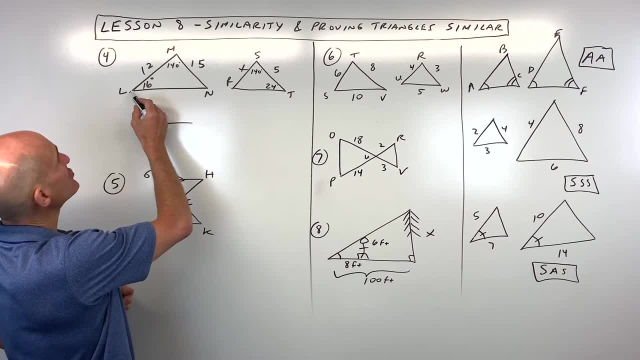 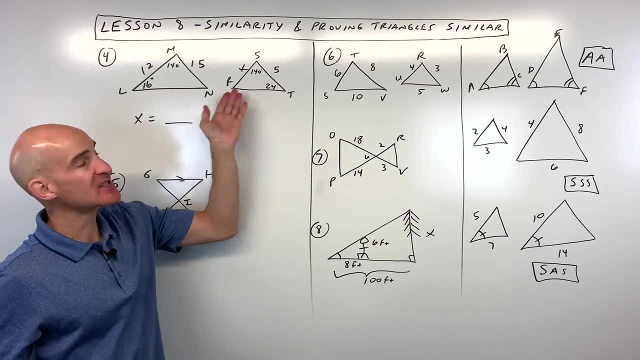 So let's go through some examples. For number four: we've got this triangle here. we've got this triangle here. The first thing I want you to do is see if you can figure out. are these triangles similar to one another? And if they are, can we solve for this missing side length here x. 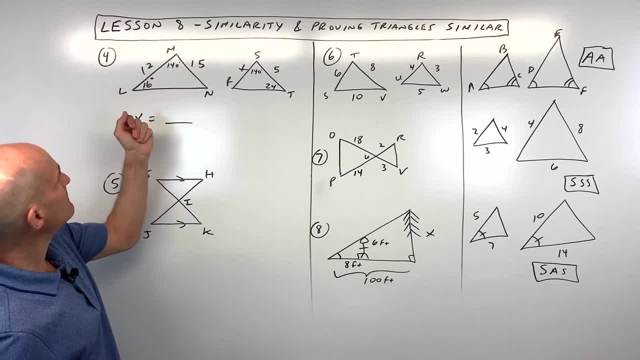 Okay, if I was going to do this myself, first thing I would do is I'd say: well, hmm, let's see what we've got here. We've got sixteen and a hundred and forty. that's a hundred and fifty-six, which means 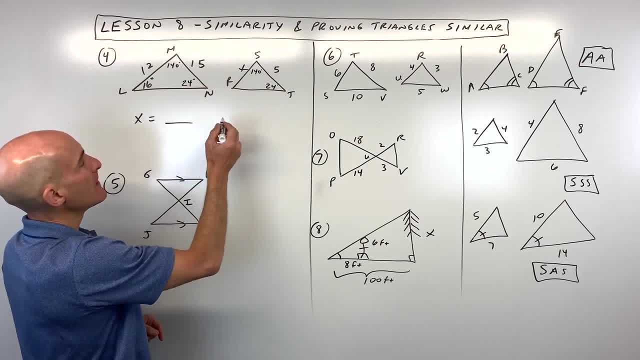 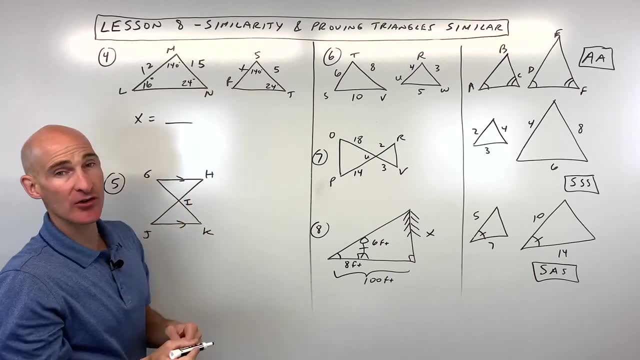 that this missing angle here would be twenty-four degrees. Over here we have a hundred and forty and twenty-four. a hundred and forty and twenty-four, oh, we've got two angles that are congruent to two angles. so we know that these triangles- 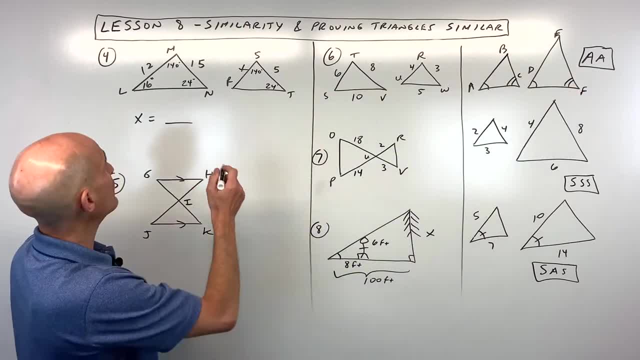 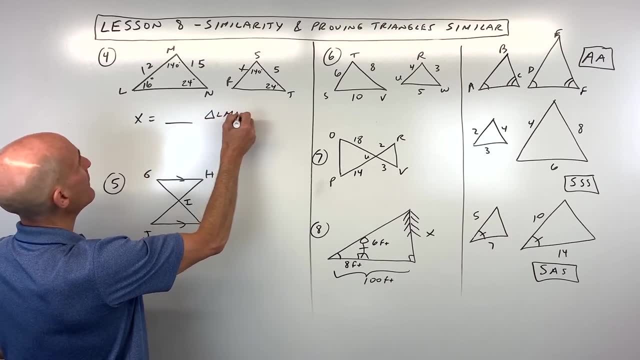 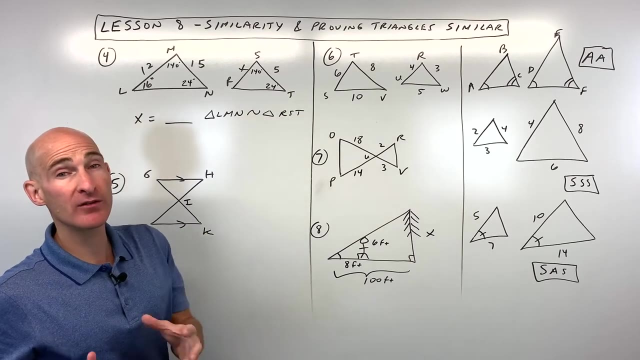 are similar by the angle-angle-single, Okay, And we can write what's called a similarity statement, just like when we wrote a triangle congruent statement. So here I would say: triangle LMN is similar to triangle RST. Now, when you write this, it's very important with the order. 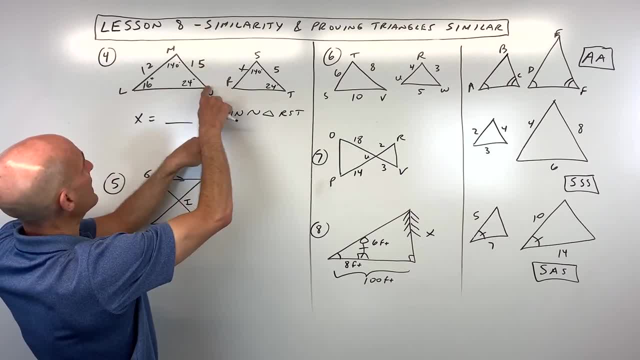 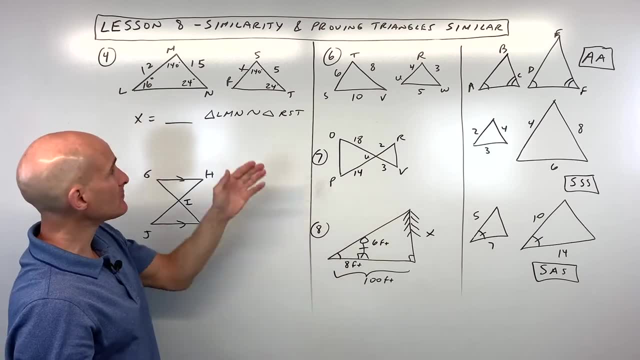 You want to make sure the corresponding vertices match up. So let's see LMN. so I'm going like from sixteen degrees to one-forty to twenty-four, to sixteen, to one-forty to twenty-four. so it's in the same order. 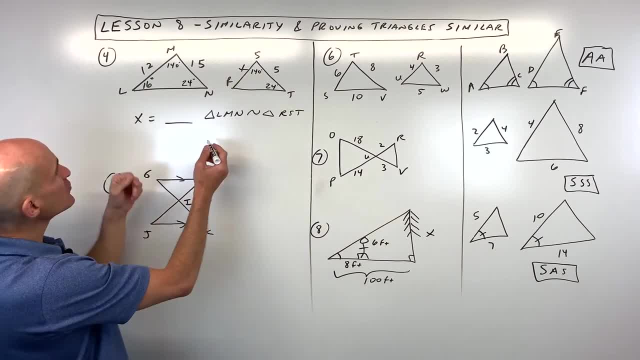 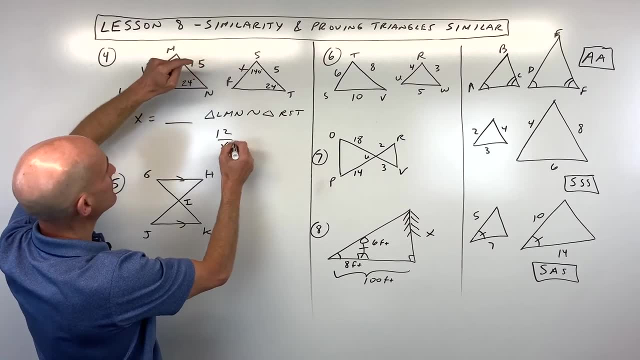 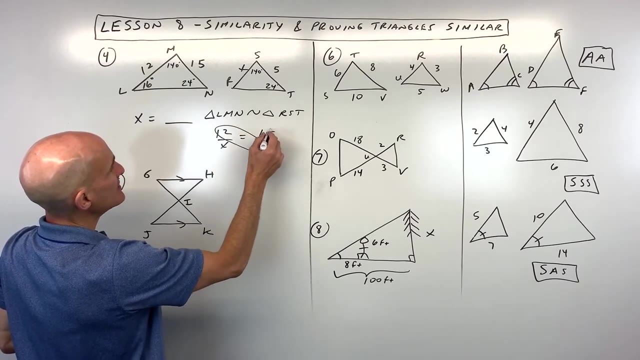 That's your similarity statement. Now how do you solve for this missing side length? Well, here we want to make a proportion, making sure we compare the corresponding sides. So I would say twelve is to x as fifteen is to five. So now let's see, we can cross-multiply. we have sixty equals fifteen, x divide both. 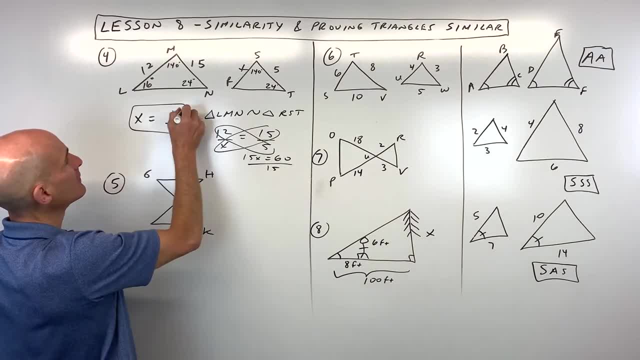 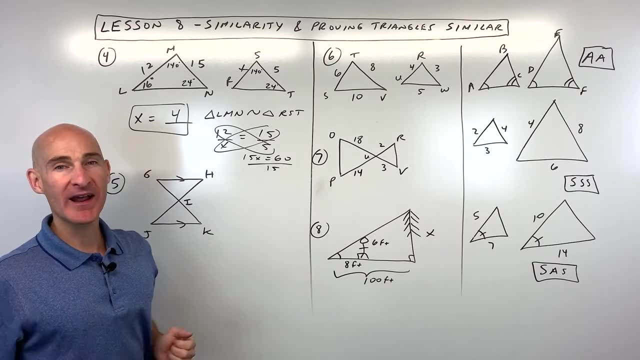 sides by fifteen, and x comes out to four. Okay, let's go to number five. now see if we can do this one. What do you think? Are these two triangles similar? Why, Why not? Hmm, Well, if I was going to do this, I always look for clues and you can see here. see, 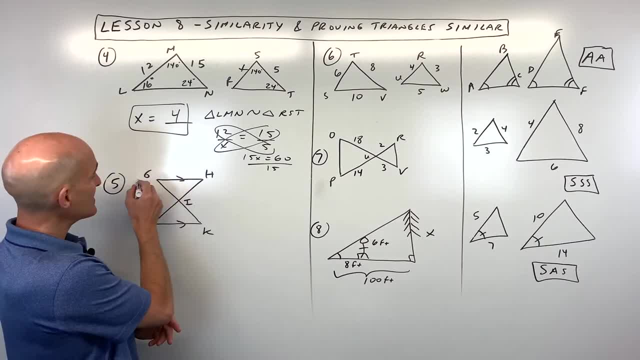 these arrows here? What do these arrows tell us? It tells us that the lines are parallel. so sometimes when I have parallel lines, I like to extend the parallel lines. You can extend this transversal and you can see, here we have alternate interior angles. 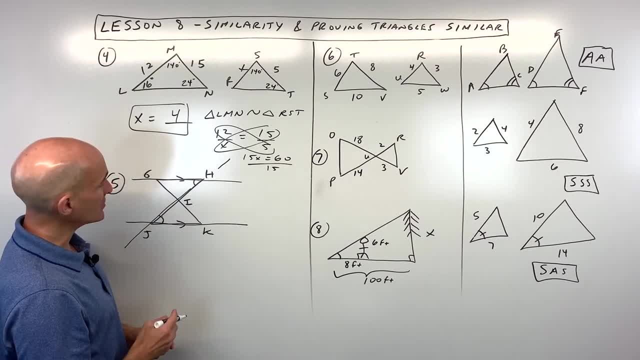 Those are congruent. Remember, from earlier on in the course we talked about parallel lines cut by a transversal and all the different angles. So we had alternate interior, alternate exterior, cross-multiply, Okay, Corresponding, etc. What do you notice about these two angles? 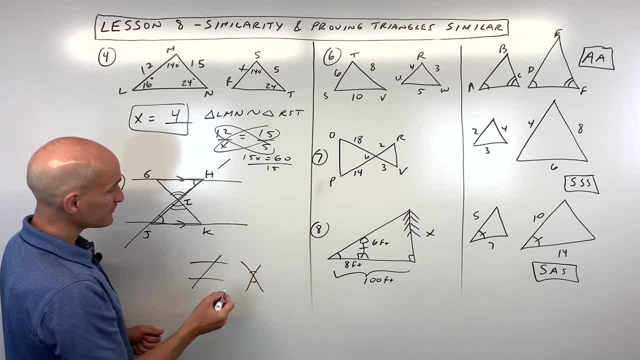 These are what are called vertical angles. see, they're across from each other in that x. So now we have two angles are congruent to two angles. so by our angle-angle similarity we know the triangles are similar. How do we write our similarity statement? 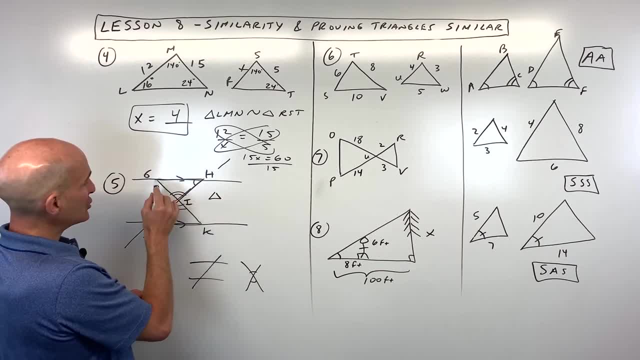 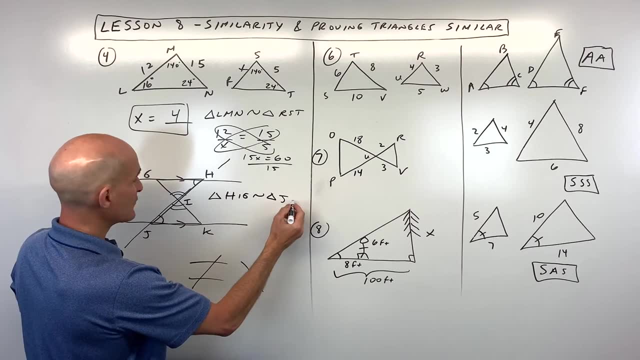 Well, we have triangle HIG is similar to triangle JIK. Now, I don't know When I was first learning about this. Uh, In school I said: well, you know, sometimes it was hard for me to, you know, turn the. 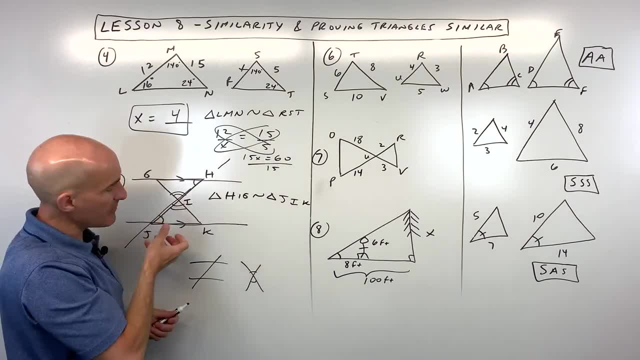 figure, Some people are really good with that. They can say, well, if I rotate it I can see how they match up. But I'll show you a little secret. You just go in the same order. See how this has one marking. 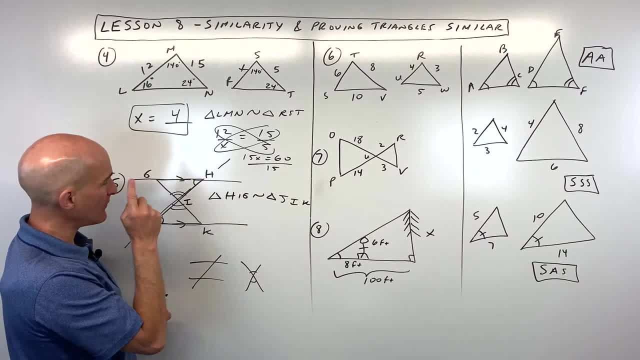 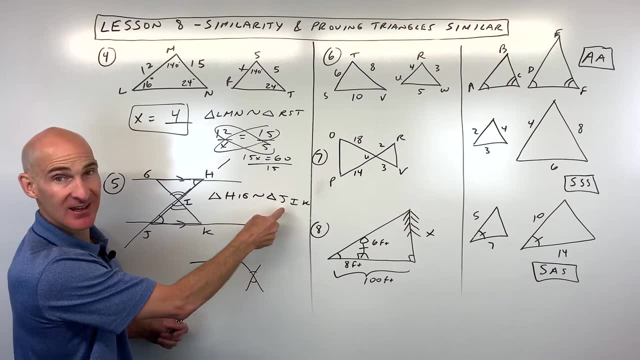 See H, I has two markings, G has no markings. So I think to myself: okay, Mario, one, two, zero, let me just follow that same pattern: One, two, zero, JIK see. Or again, you can kind of rotate it and match them up. 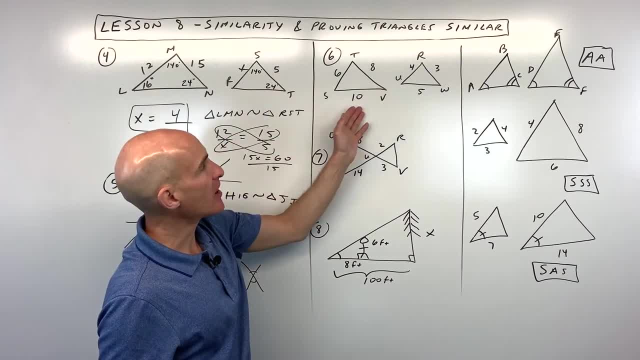 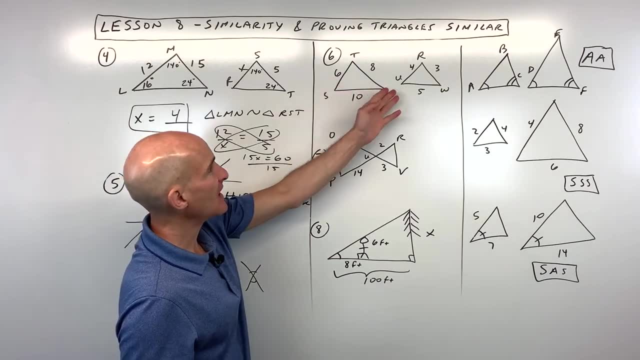 So that was angle-angle. So for number six, what do you think for these two triangles? Are they similar? Why or why not? And what would the similarity statement? how would that be written? Well, let's see, It doesn't look like they're giving us any angles here. 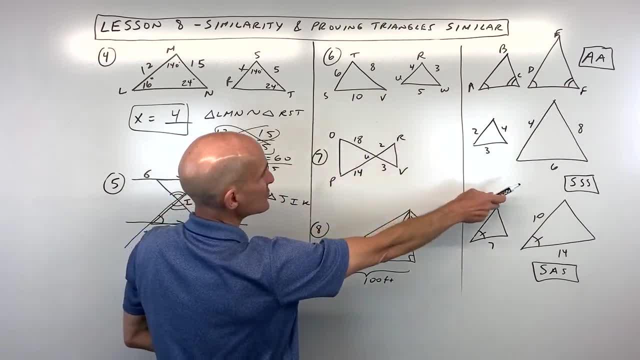 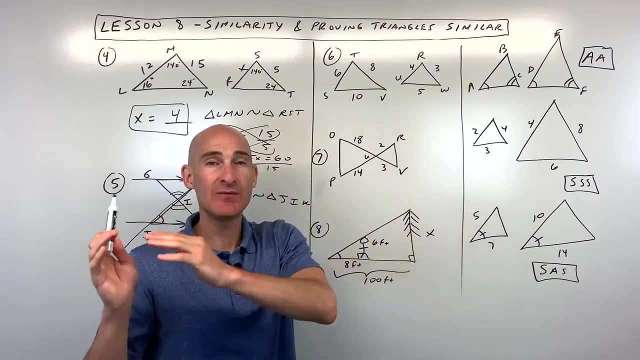 So we probably can't use that angle-angle. We do have three sides so it might be side side side. The key here with side side side is you want to make sure you match up the short side with the short side, the medium length side with the medium length, the longest with the. 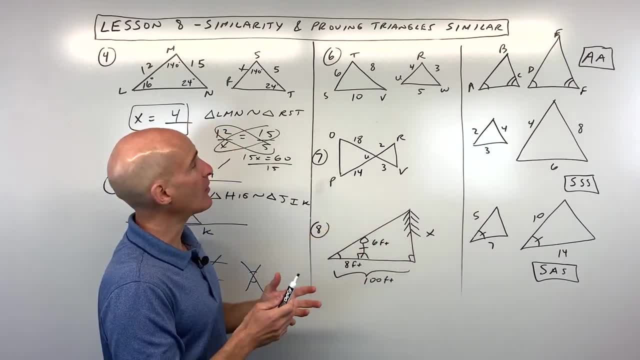 longest. If you don't do it in that order, you know they may not work out. So you want to compare them? So let's see. Three is the shortest over here, Six is the shortest over here, So let's see. 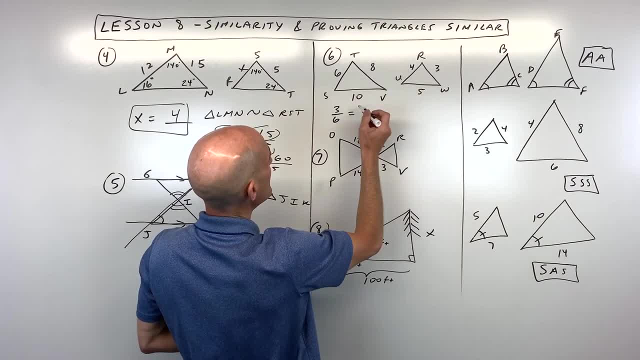 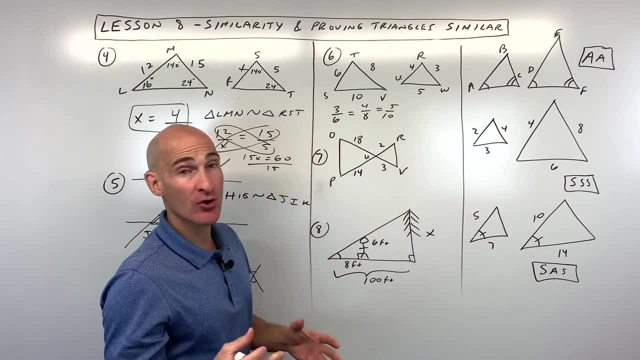 Is three to six, the same as medium to medium. That would be four to eight. How about the longest here to the longest here? Yeah, it looks like that's one half, one half, one half. Okay, so they're all in the same ratio. 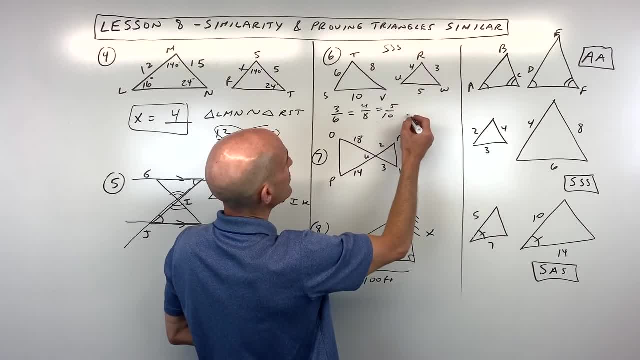 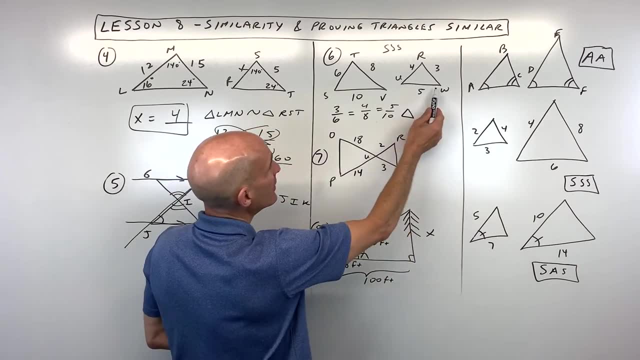 So they are similar by the side side side. And let's write our triangle congruence, not congruence, our triangle similarity statement. This would be triangle. Let's see Now watch this pattern: Short side, medium side, long side. 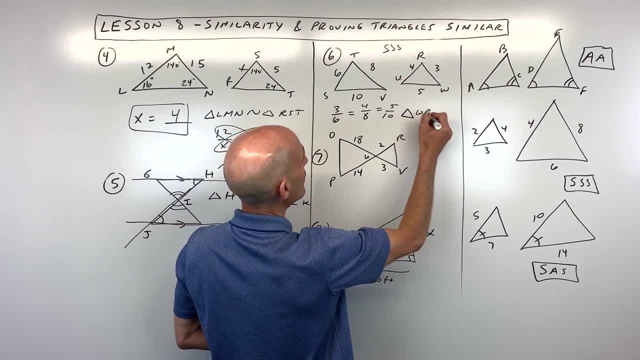 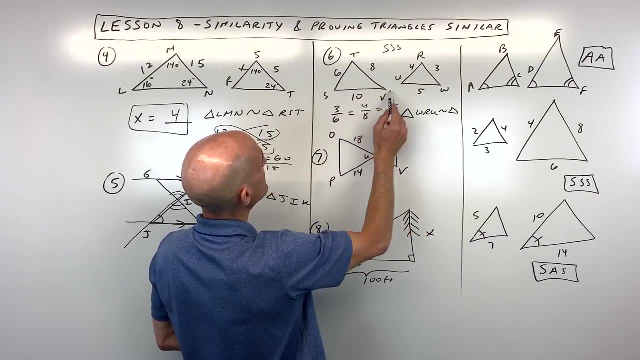 So that's W R U back to W right. W R U is similar to triangle. Let's keep that in the same order when I do short, medium long, So we're going to do short, medium long, S T V. back to S S T V. 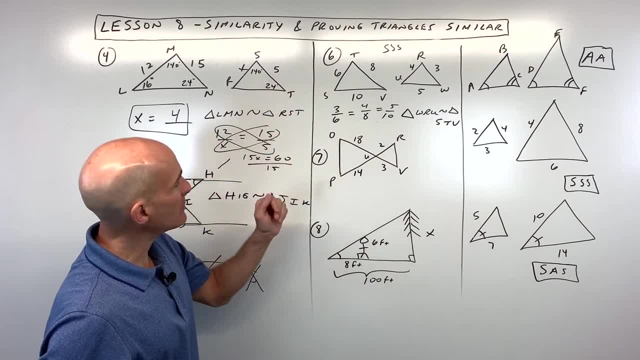 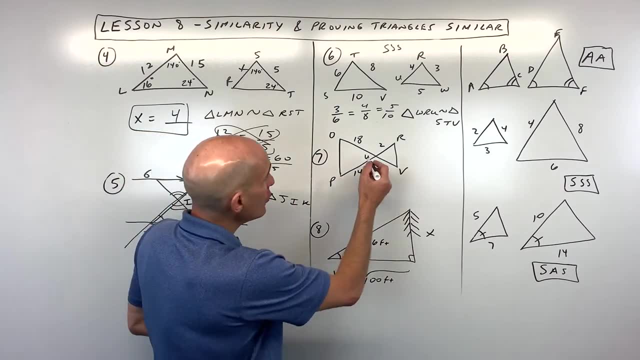 Okay, good, So that was side side side For number seven. what do you think for this one? Are these two triangles similar? Well, we don't have any angles again. However, we do know that these angles are congruent by vertical angles. 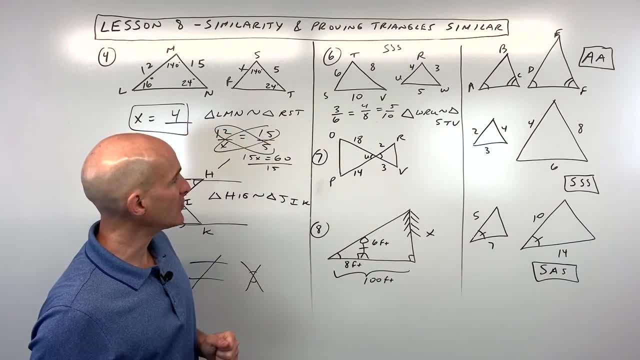 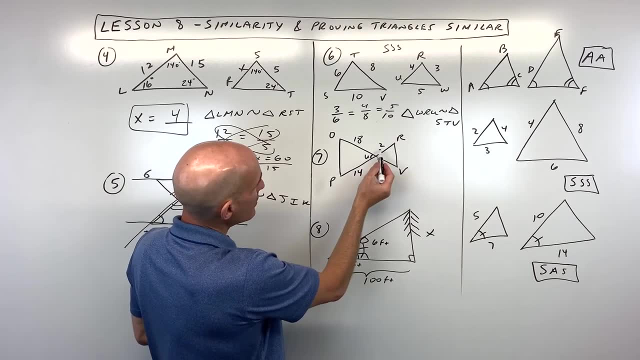 See that X that's formed, The angles across from the X, The X are congruent by vertical angles And it looks like we could have side angle side. See how the angle is in between the two sides. So again we want to compare short side over here to the short side over here. 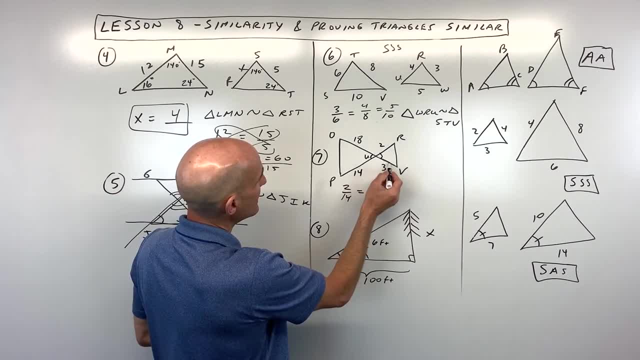 So is 2 to 14 the same as the longer side here to the longer side here, 3 to 18?? Well, let's see, Let's reduce. That's 1 to 7.. Is that the same as 1 to 6?? 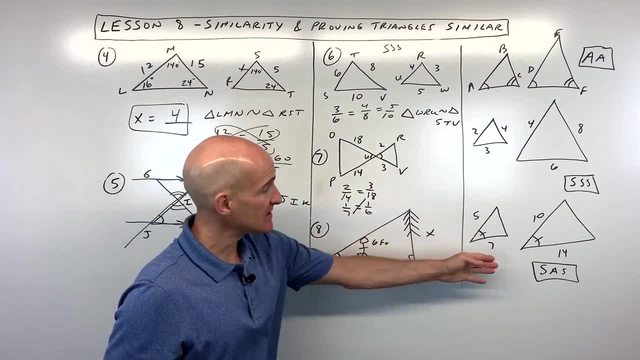 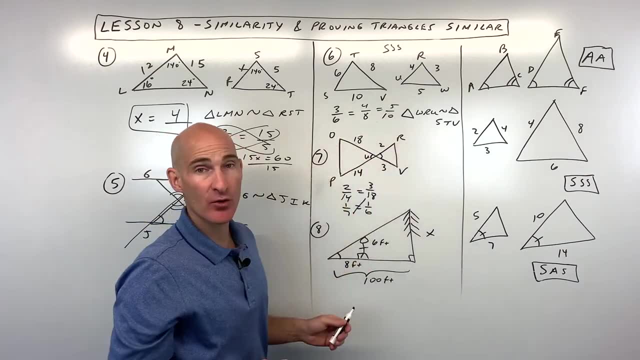 No, So this one is not actually going to be similar by the side, angle, side similarity If they were both 1, 6 to 1, 6.. Then again, you know you want to make sure you rotate it to match up the corresponding. 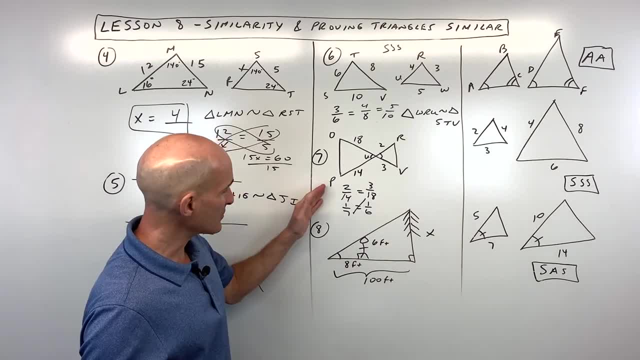 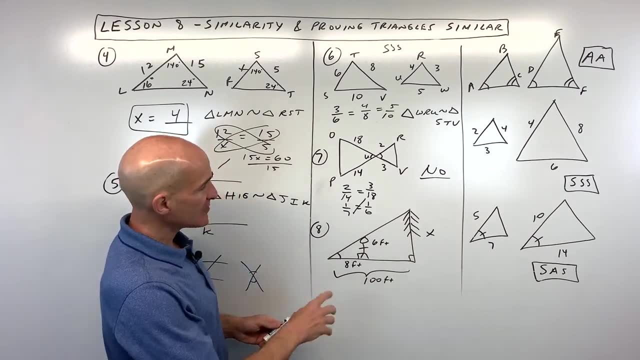 sides and the corresponding angles, So that one was not similar. And for number 8, this is kind of like a real life type of problem, Like say, for example, you know, the sun is over here up in the sky, right. 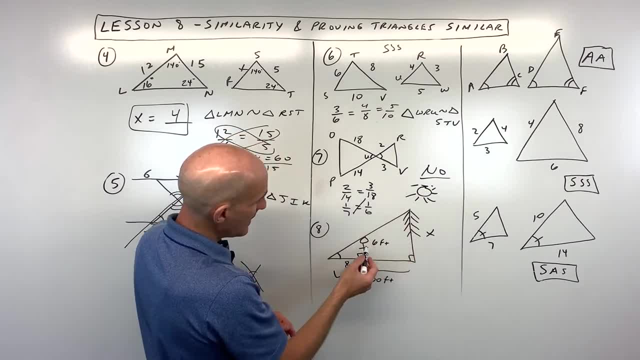 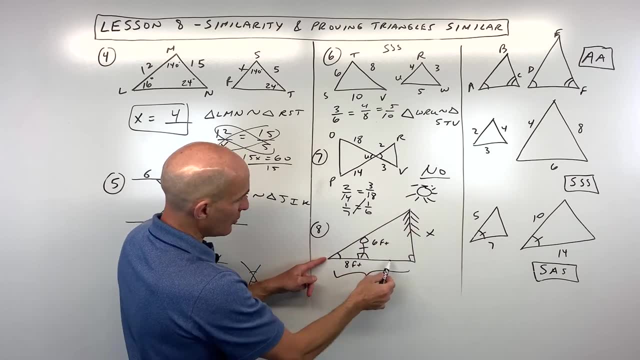 And here you have a tree and you say: I want to figure out how tall is this tree? And let's say you're six feet tall and it casts a shadow right here. Okay, The tree is also casting a shadow, okay, along the ground here. 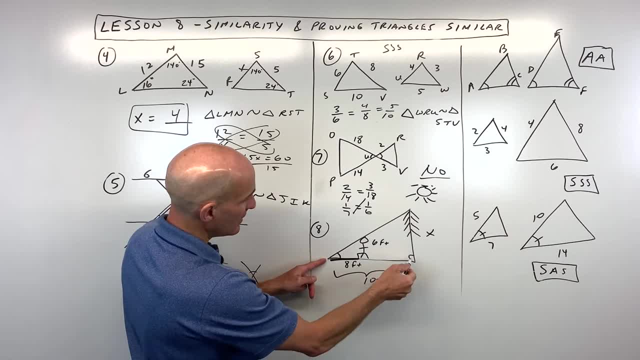 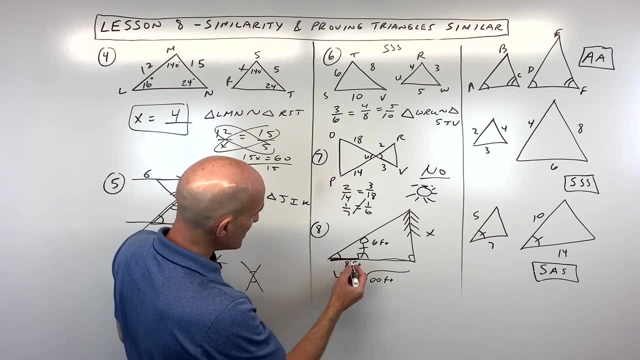 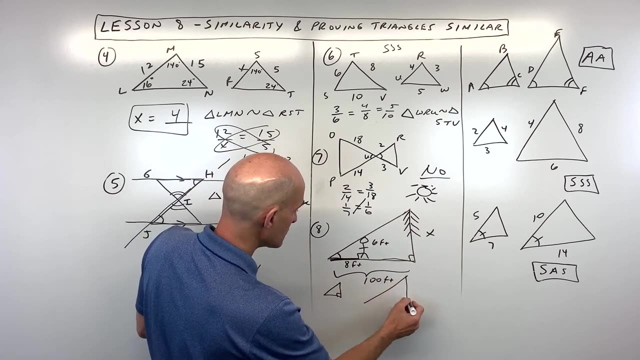 And the shadows: they coincide, Okay. So here's your shadow, Here's the tree's shadow, And so what we have is we have two triangles. Sometimes it's helpful to draw the triangles separately. So say this little triangle right here. say this whole triangle right here, okay. 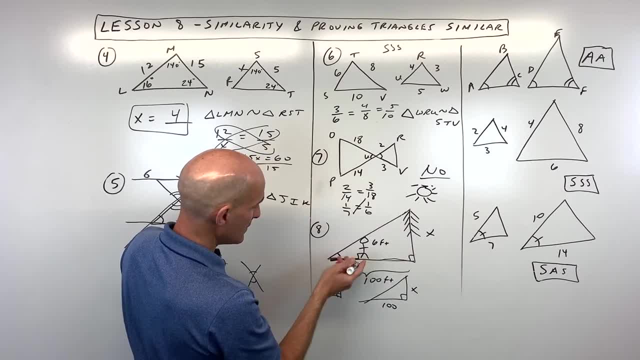 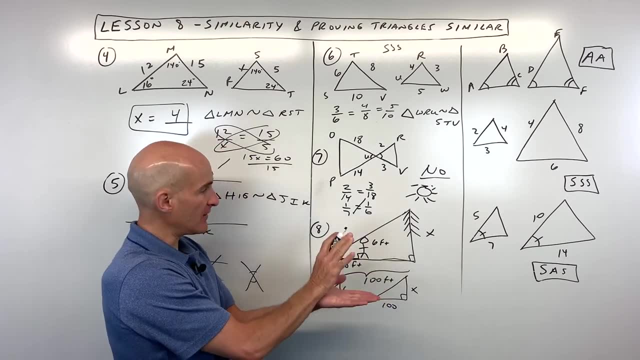 And so we have X and 100,. okay, 100 feet, We have six feet is how tall the person is, And here's their shadow: 8.. And notice this angle- here We call this the angle of elevation- okay- to the sun. 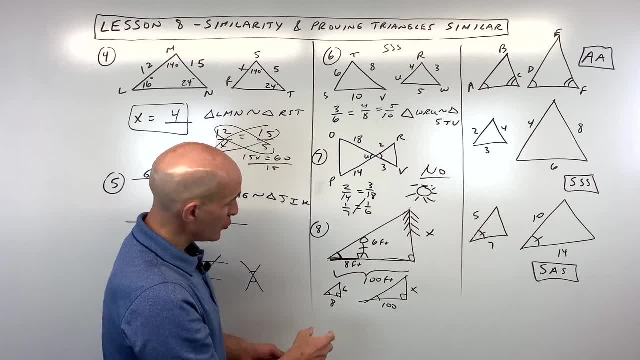 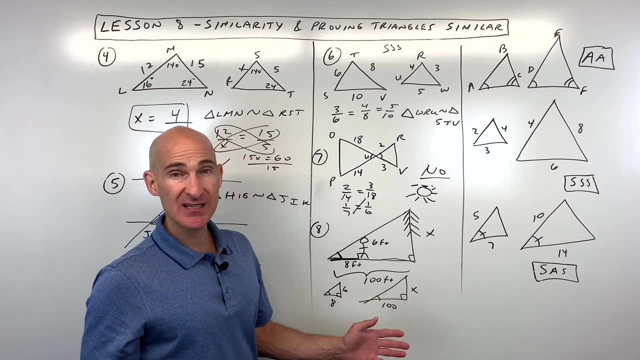 That's going to be the same here for the person. as to the tree, Notice we have angle angle. See, two angles in one triangle are congruent to the two angles in the other triangle. We know the triangles are similar, which means the corresponding sides are proportional. 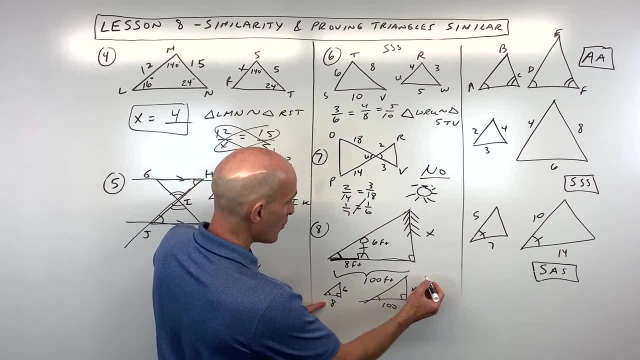 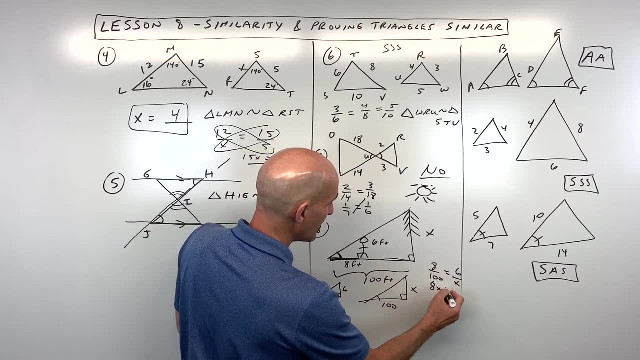 We just have to make sure we match up the corresponding sides. So 8 is to 100, as 6 is to X. Cross multiply We have 8X equals 600.. Divide both sides by 8.. Let me go to the calculator on this one. 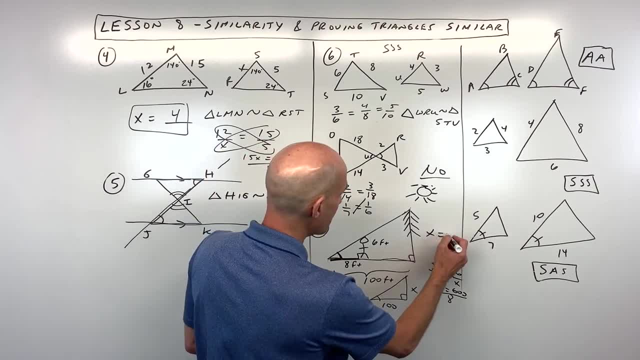 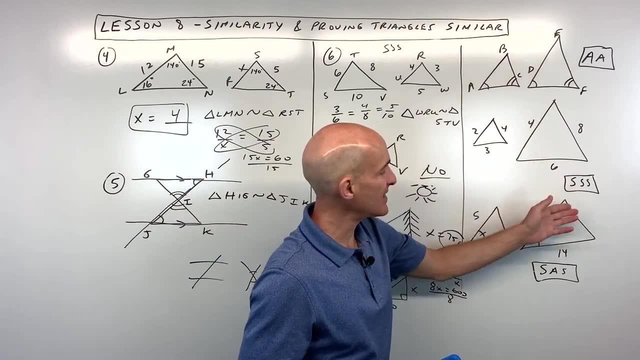 And it looks like it's going to be 75 feet tall. That's how tall the tree is, And you got it. So similar triangles, three methods: angle angle side, side, side side, angle side. Okay, now we're going to talk about a few more theorems here. 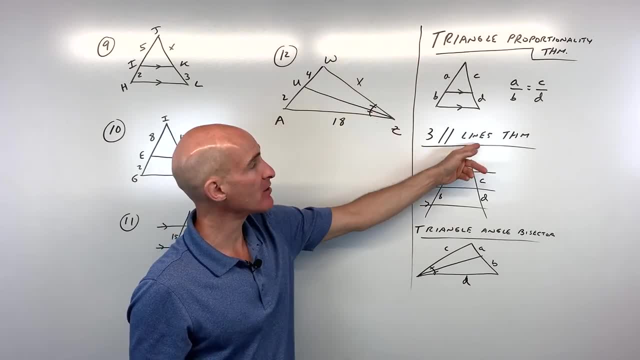 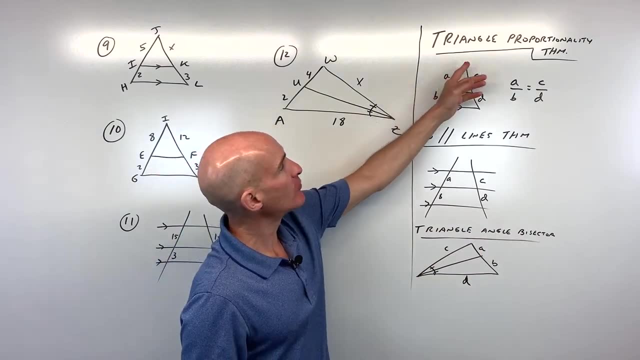 We've got the triangle proportionality theorem, the three parallel lines theorem and the triangle angle bisector theorem. So what are these all about? Well, the triangle proportionality theorem is when you have a triangle. And if you have a triangle, 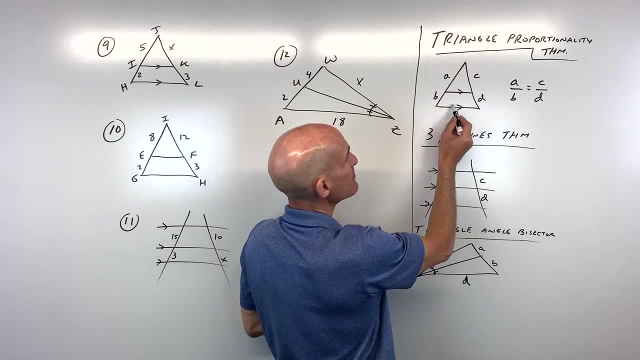 And if you draw a line or a line segment such that it's parallel to the base, what it does is it splits up these two sides into two segments- see A and B, C and D, And there's a proportion that's formed. 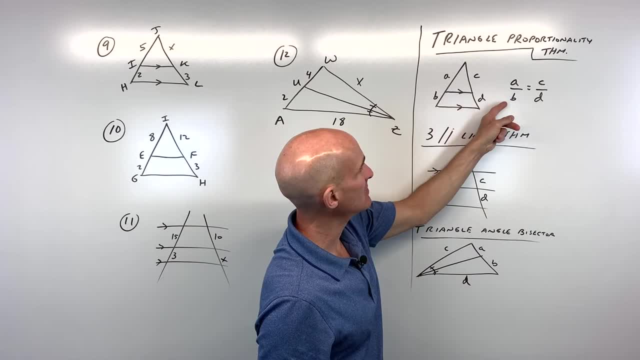 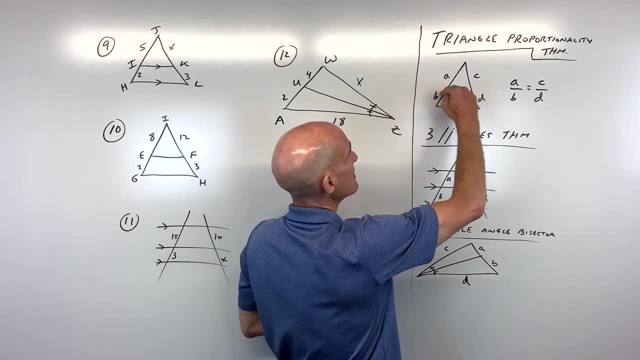 The ratio of A to B is the same as the ratio of C to D. okay, So sometimes it's referred to as the side splitting theorem, because this line here, this segment, it splits the two sides into two segments And the ratio is going to be the same. 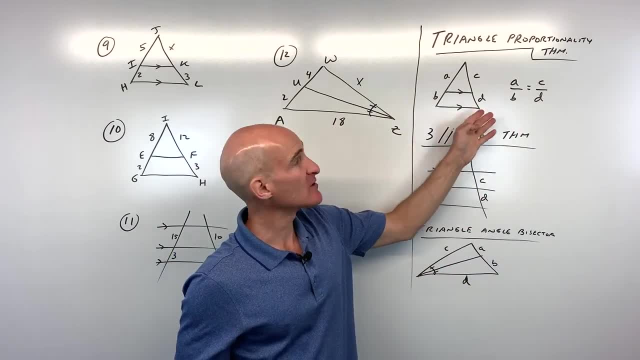 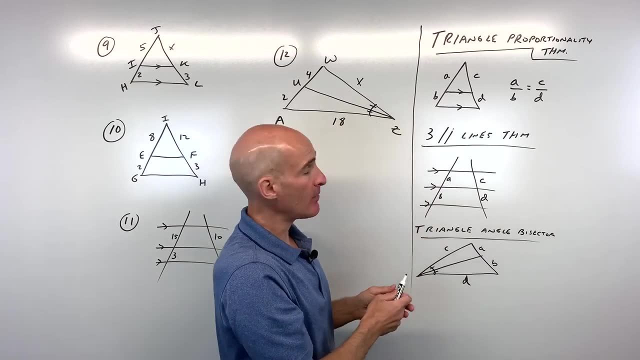 So you can form a proportion Now with the three parallel lines theorem. it's very similar to the triangle proportionality theorem. You have three parallel lines which are denoted by these arrows, So we know they're parallel, And a transversal transverses or cuts across those three parallel lines. 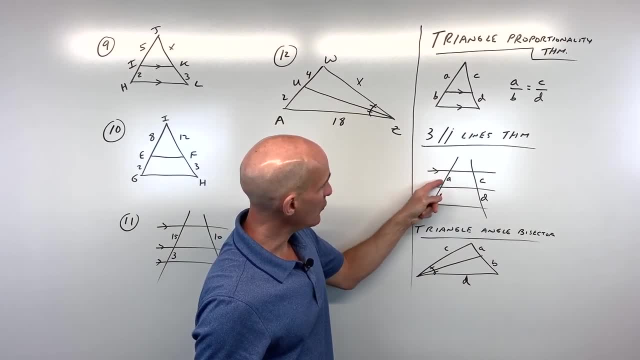 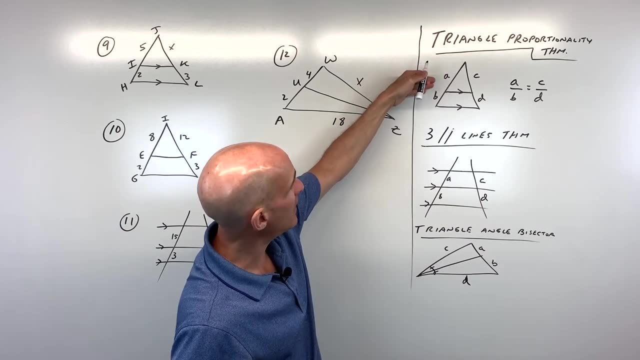 And you can see that there's these segments that are formed. The ratio of A is to B is the same as the ratio of C is to D. You can kind of think of this as your triangle. You can think of the triangle proportionality theorem, and imagine if you put a third line. 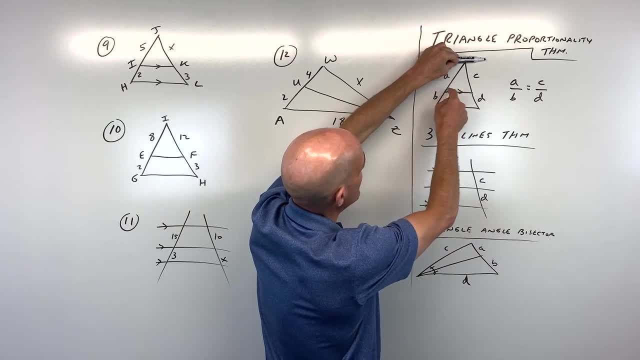 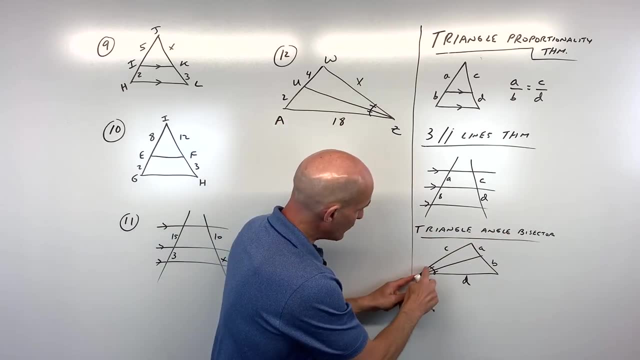 here at the top that's parallel to these two lines. you have that same ratio: A to B, C to D. And then the last one, the triangle angle bisector theorem. you have a triangle and one of the angles is bisected, meaning cut in half. 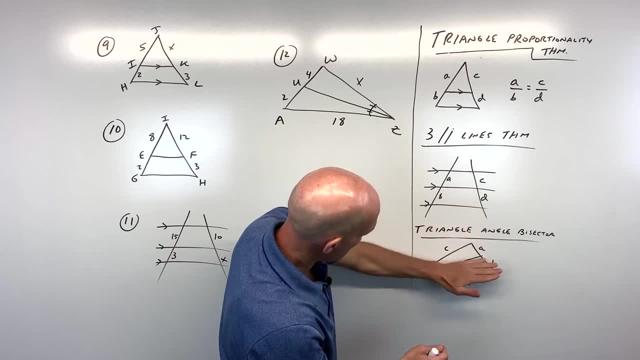 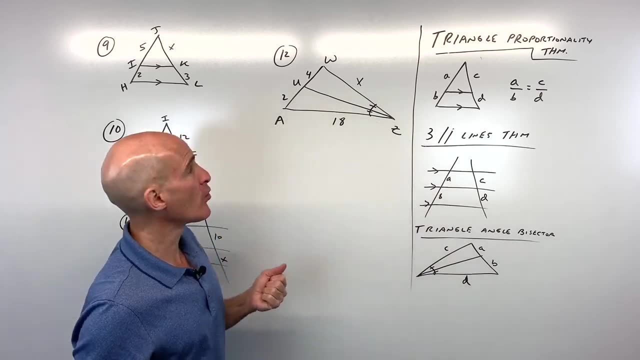 And you can think of taking this top triangle and folding it, okay, onto this bottom triangle. like this, The ratio of A to B is the same as the ratio of C to D. Okay, so we're working with these proportions. I'm going to use these angles just to show you how this works. 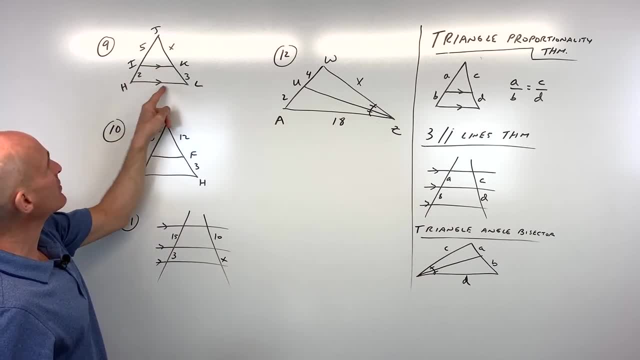 So say for number 9, here you can see that this segment is parallel to the base. So we know that it's the triangle proportionality theorem. We know the ratio of this segment to this segment is the same as this to this. So let's go ahead and set up our proportions. 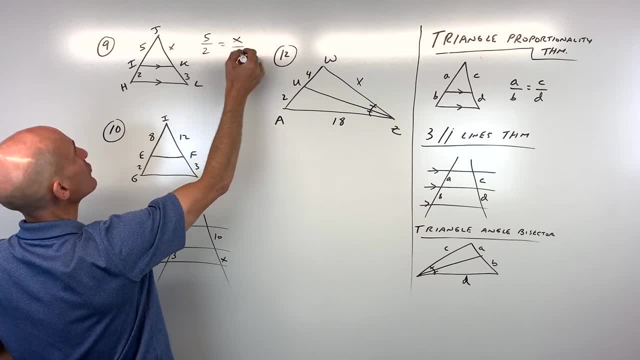 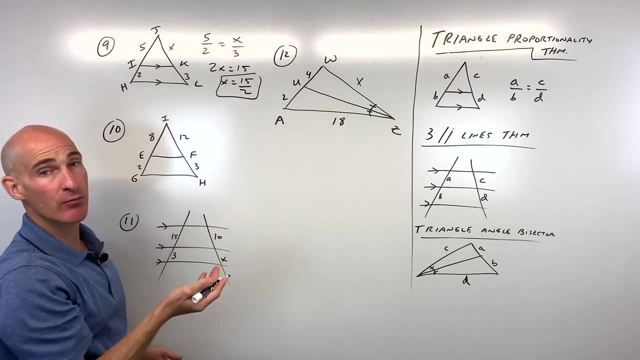 So 5 is to 2 as x is to 3. We cross, multiply, We get 2x equals 15, and divide by 2. So x equals 15 halves or 7.5.. For number 10, this one's a little bit different. 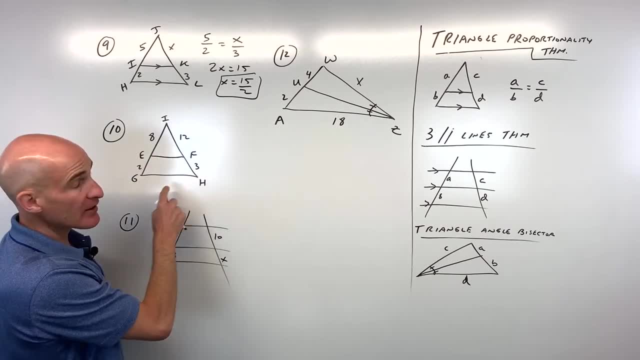 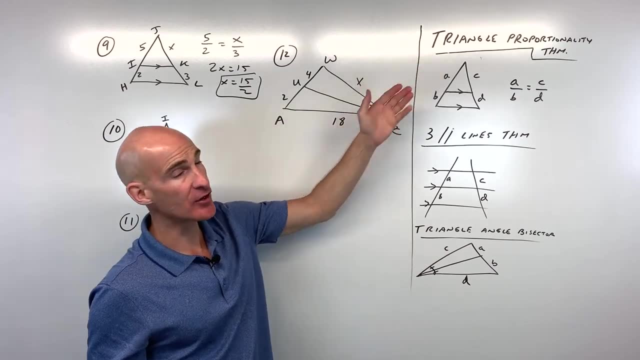 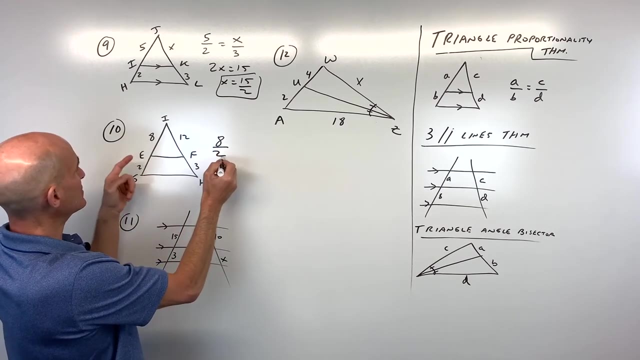 The question here is: is EF parallel to GH? So is this segment parallel to the base? Well, that's the converse of the triangle proportionality theorem. It's like saying it in reverse or backwards. And the only way that this would be parallel to this is if 8 is to 2 is in the same ratio.